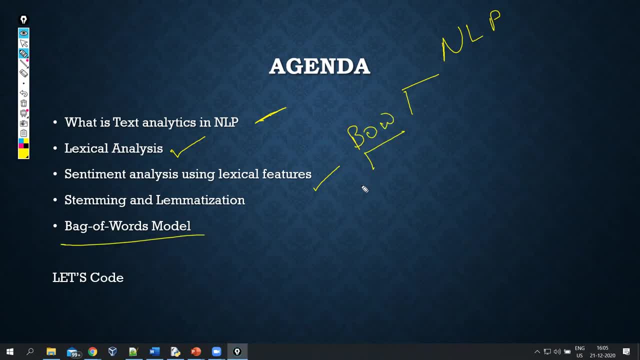 model. Okay, so we will see what is this bag of words model, completely with theory as well as with coding, So you will know in depth. So, starting with this, I would start with first thing, like, in short, I will explain you what is NLP, So you might have heard about, so everyone. 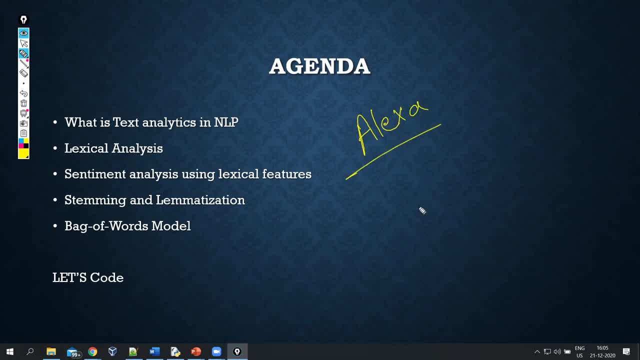 else you have heard about Alexa. Okay, so what has made Alexa such in a boom in the market? So there are multiple speakers, some optionizers, Apple and many other brands are there, but why Alexa came to the boom? You can give me your answers. 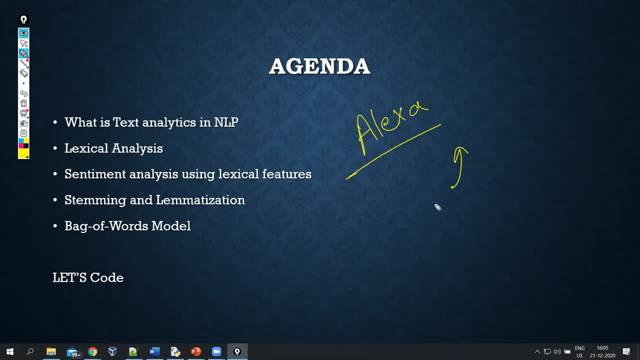 Okay. So yes, I hope everyone is able to make a right guess like, yes, like you said, natural language, like Alexa, is able to hear you and respond you okay. This makes Alexa different from any other speaker, for example, JBL, If a JBL speakers, So you can say Alexa that hey, Alexa play some romantic songs of Shahrukh. 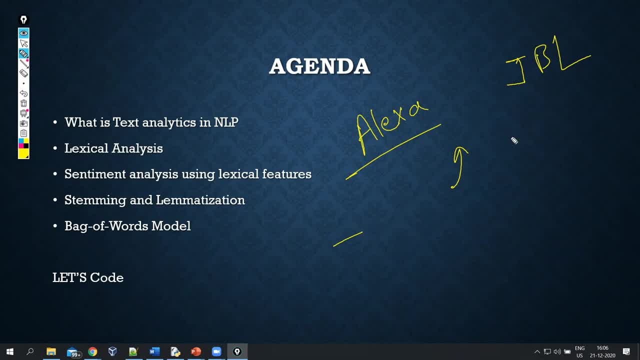 Khan, but you cannot see the same thing to JBL. It cannot understand that, So is able to interpret your language and give you the result back. so in order to interact with JBL, you need some interface. might be your phone touch screen or trackpad or keyboards, anything. 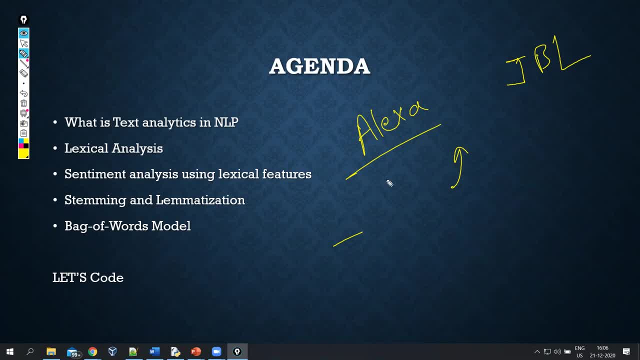 you need to use some interface to remove this interface barrier. that is, to naturally communicate with the machine is called as natural language processing. so, in short, like you communicate with your siblings, you directly speak to them or any other human, you speak to them, so that is your. 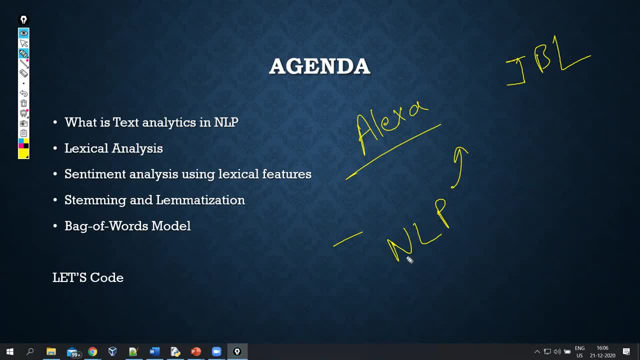 natural language. now, to make machine understand your natural language, this NL, we need to do some processing, that is, natural language processing, so your speech is understandable, that is, your natural language is understood. now to Alexa: it can understand it, interpreted that he you want some romantic songs of Shah Rukh Khan, and it can make actions based on that. it can even reply you. 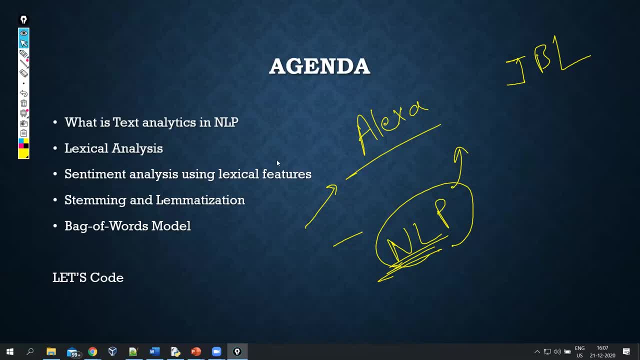 in the form of human, so that make Alexa stand out from different speaker. this capability is possible due to NLP, so NLP is just understanding a natural language. so natural language can be gesture recognizations- like you can do gestures, and human can understand you. you can give that ability to computer as well. 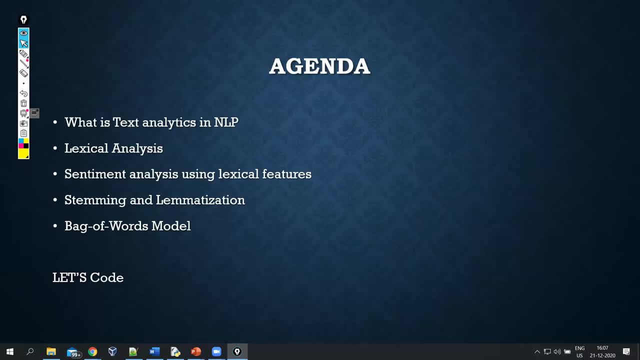 or sentiment analysis is one part of natural language processing. like, whatever you are saying, your sentiments, whether you are positive, negative, harsh, rude, anything, it is clear to other human. so machine can understand your natural language. so that make Alexa stand out from different speaker, except human, that we can distinguish. the你們 can be the same person. you know amazing can also. 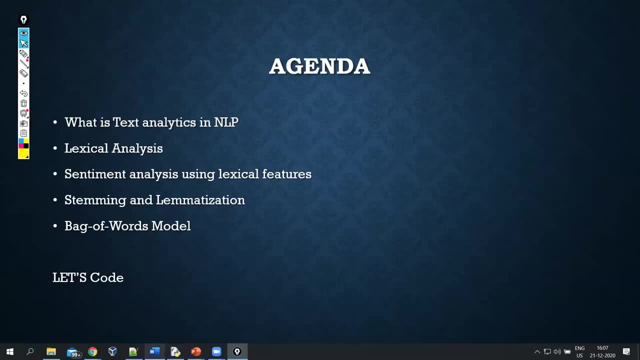 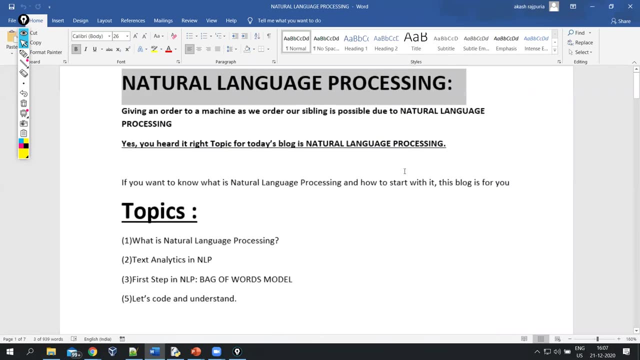 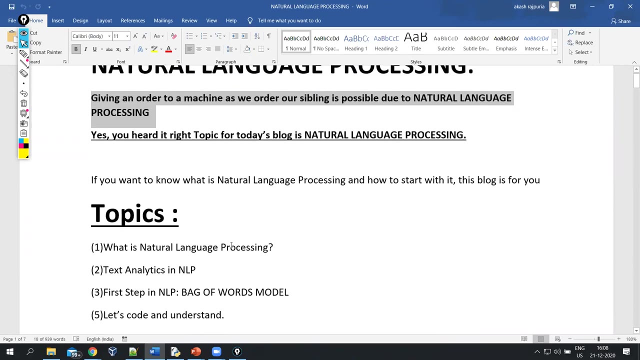 understand it. yeah, with the help of NLP. okay, so that was a basic Indicator. introduction of NLP, that is, natural language processing. giving an order to machine aZ- we order our siblings- is possible due to natural language processing. likely. you order to a simple alexa, okay, so like in this: 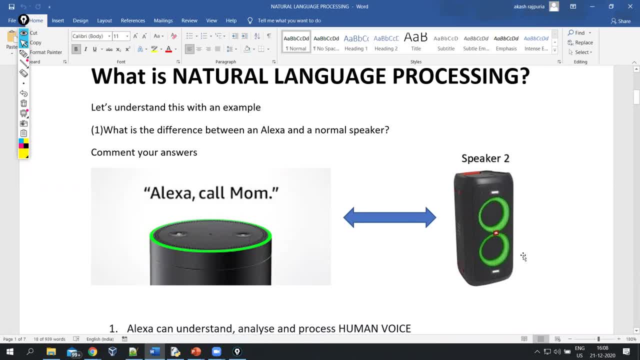 way you can say: Alexa, call mom. but you cannot say to the second speaker: I like second, understand, analyst human voice so Alexa can understand the human voice. the необход of human language useful to use voice can analyze human human voice. same with Alexa: we understand Braille and weather often. 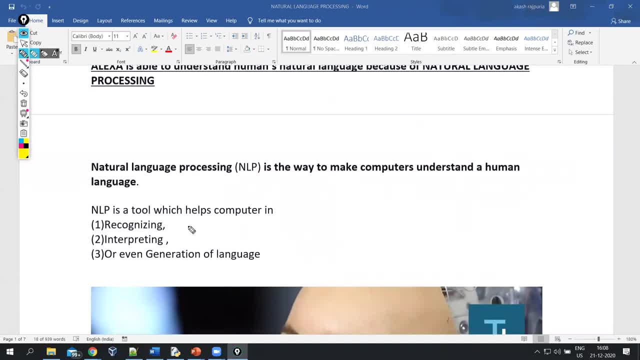 Okay, so like in this way, you can see alexa call mom, but you cannot say through to this second speaker. Alexa can understandionalize human voice same way in. In short, NLP is consisting of three things. Like I said, it would recognize your voice. 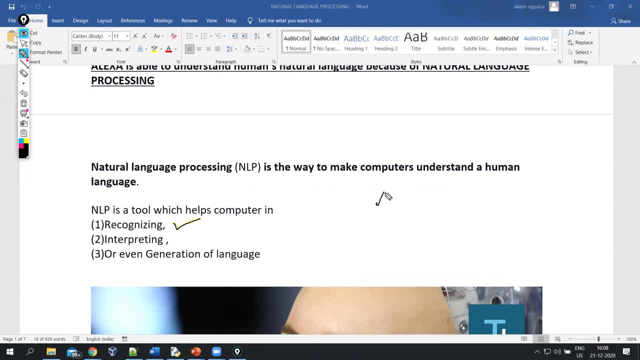 After that it will interpret it. So your voice isn't in the speech forms something like this. So it needs to recognize this, then interpret it. Interpret means that understanding what you want. You want romantic songs. That is interpreting, And after that even generation of language. 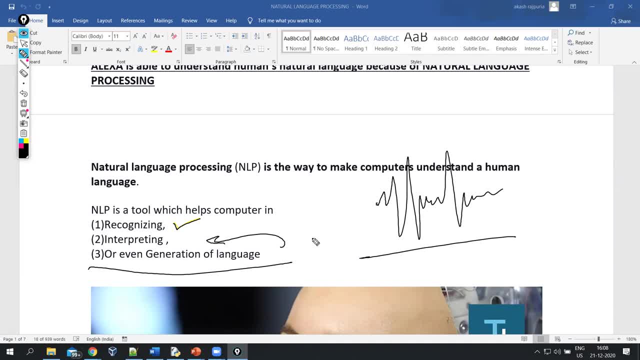 So Alexa can speak also. That is the three major tasks of NLP: to understand and communicate as a human. In short, NLP is a way to make computer mimic like a human, Like you have heard about this Sophia robot, which has been awarded with a citizenship. 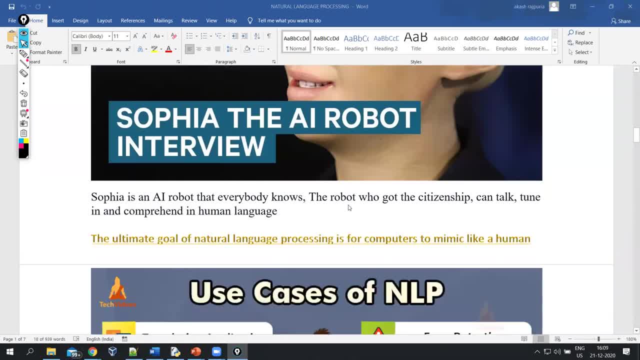 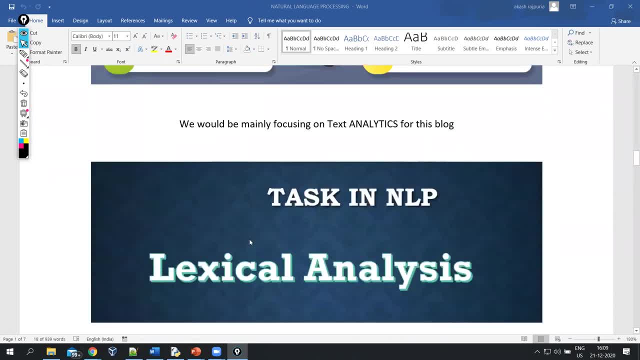 So that can tune and comprehend like a human. Ultimate goal of NLP is make computer mimic like a human. So there are multiple use cases in NLP. We will only focus on one thing, That is, there are multiple domains. Like I said, speech is one domain. 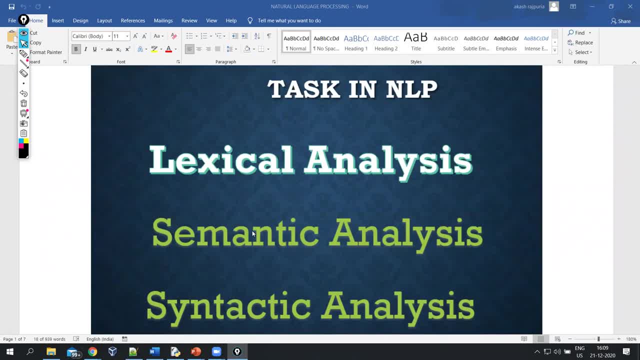 Text is one domain, Gestures are one another domain And there are multiple, But in this lecture we would only focus about text. So this is the major part of the text. So I hope everyone is clear up till now. If you have any doubts, you can stop me at any point and let me know. 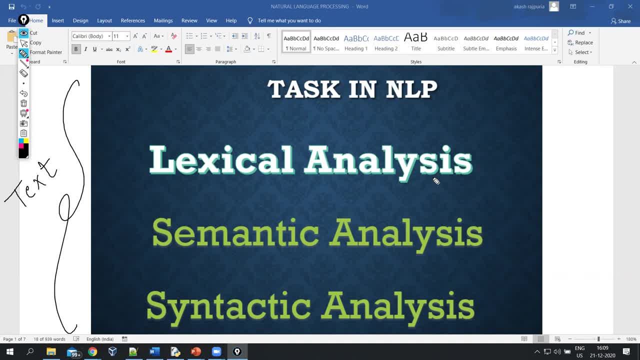 Is it clear everyone up till now? Great, We can start with text analytics. Now, a text is something a machine cannot understand. Machine needs, we need to make machine understand the text. That is why text analytics. So in text analytics we have three things like lexical, semantic and syntactic. 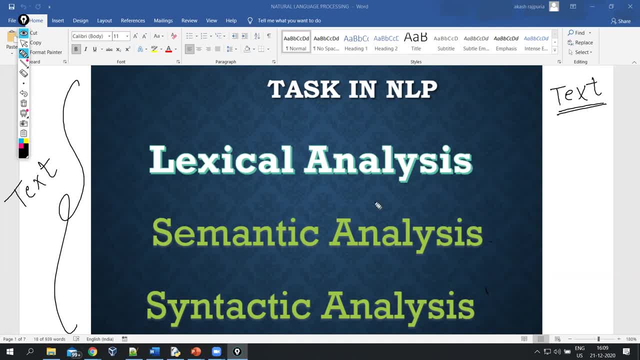 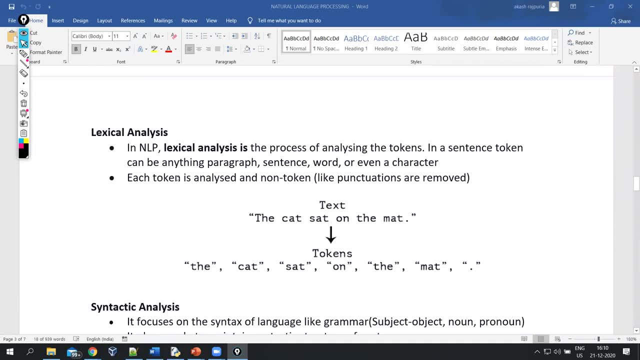 Only the naming is difficult, while everything in that is very simple. So we will see this step by step. like the lexical analysis, So lexical is the first step in text analytics, which means that lexical means breaking your sentence into tokens. Okay, breaking any things into token. now, in text, token can be anything. 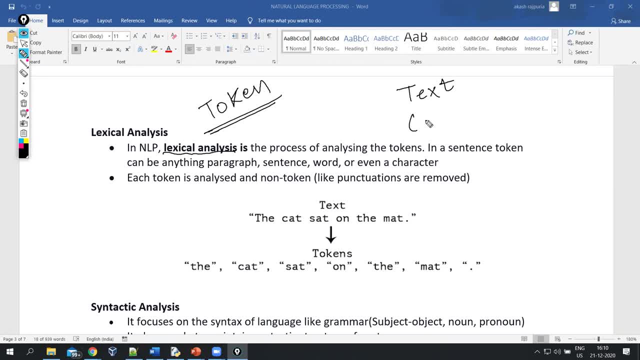 So understand this. So text is text can be a complete paragraph. Like I like this food, Full stop Food is best. These are two sentences separated by full stop. Now token tokenizing or lexical analysis means that in lexical analysis, process of analyzing the tokens, 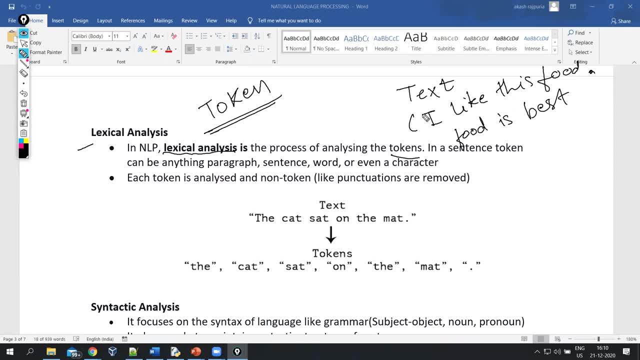 So now, what are tokens? Token is the smallest part in text or smallest part, or you can say that breakdown of text, So this text can be break based on sentences. So this can be one token. This can be another token in this with two tokens, or you can further divide it, like each word can be a token. 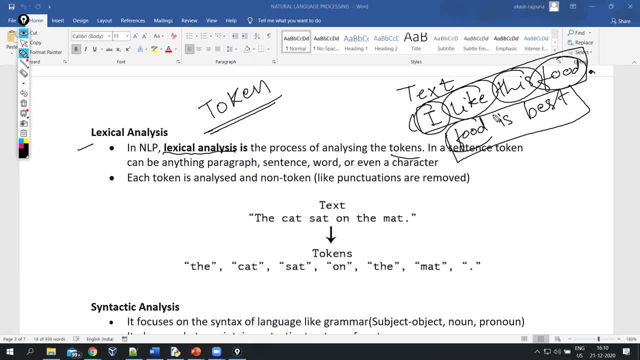 Like, as I said you, each word can be the token and you can further divide it. like each word has characters, like the word like has character L, I, K, E. So it depends. whatever is your situation, Your tokens may change, But lexical analysis is analyzing the token. 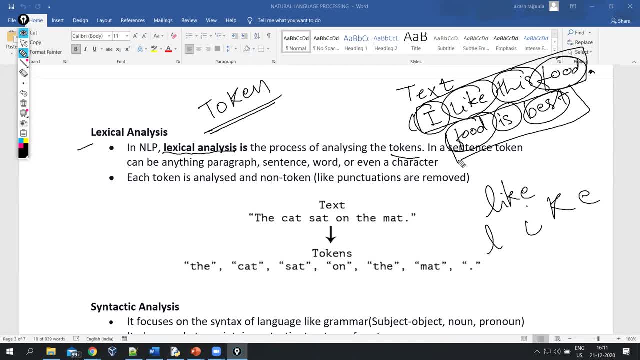 So tokens can be a character word, sentences or even the complete paragraph. So if you have a paragraph or if you have a word document of 10 paragraphs, so each paragraph can be a token. So that depends what took, how you want to analyze the text. 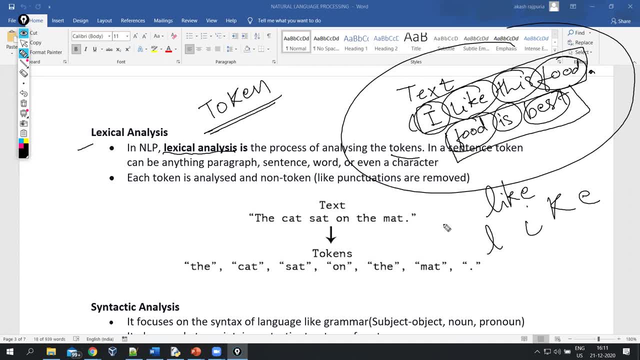 So lexical analysis is analyzing the token. But by default token are words. Okay, so to make it simple, whatever is your text, Each word is the token. And now it also consider this punctuation. So for computer, this punctuation are not different. 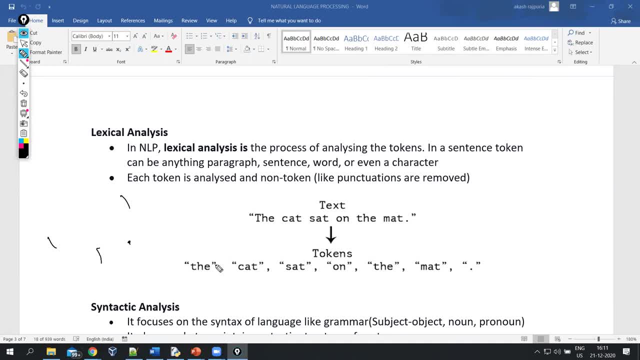 But we all know that this punctuation are different from the words, So we remove that punctuation. basically, while understanding the text that depends on domain to domain. for about for this assignment, We will remove the tokens, non-tokens, like punctuation and all other things. So basically, lexical analysis is simple: breaking down into tokens and analyzing the tokens in sentence. 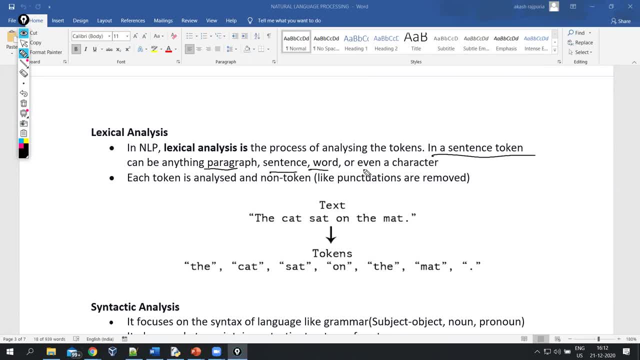 Like I said, token can be paragraph, sentence, word or even character. So now this is your complete sentence. The token can be the cat set on the mat, and even this full stop. So we will, at the end, remove this punctuation. like you know, in English, 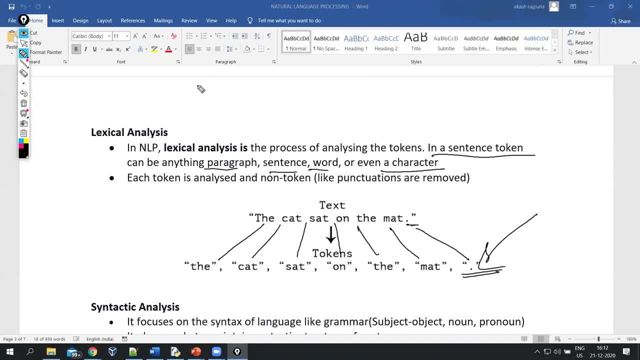 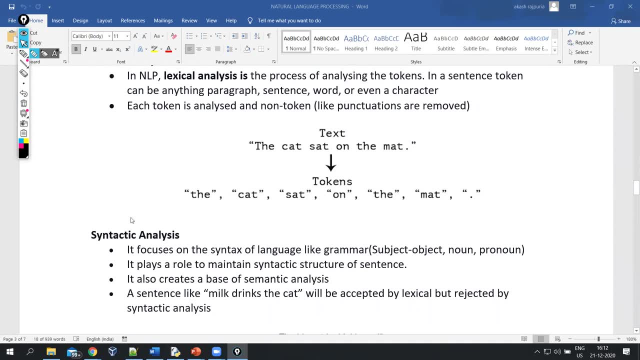 So now this was all about lexical analysis. Same way, syntactic is a next part of it. Now in syntactic it, like the name suggests it, focus on the syntax part. Like the name is syntax. So in while writing English you need to focus on the syntax, like a subject would be there and then there would be object. 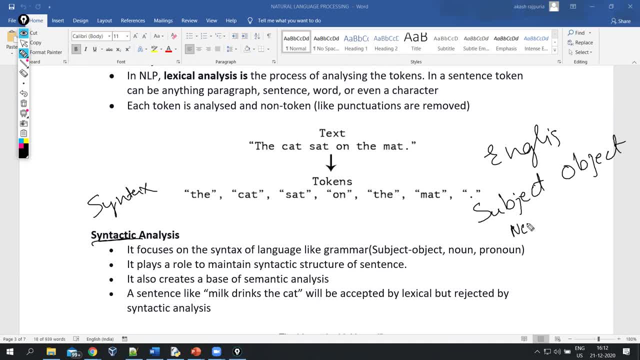 In this way. there are some rules. then there are rules like noun should be used, pronoun and all other things. There are the rule that is called a syntax. So basically, syntactic analysis, focus on syntax of the sentence Like, for example, milk drinks the cat. 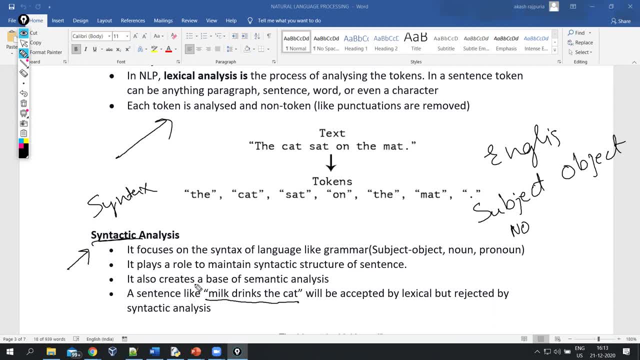 So if you break that and do the lexical analysis on top of it, So lexical analysis would be: milk drinks the cat. So this all are the four right words. So they would be accepted by the lexical. They would be accepted by lexical But may be rejected by syntactic. 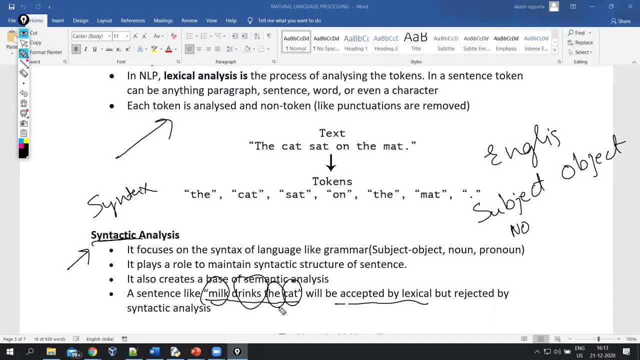 Because you can understand. the sentence is not syntactically right. The cat should be first and the milk drank. the milk should be at the end. So, syntactic, focus on the syntax of the sentence. It is clear up till now, Like it. focus on the cat. 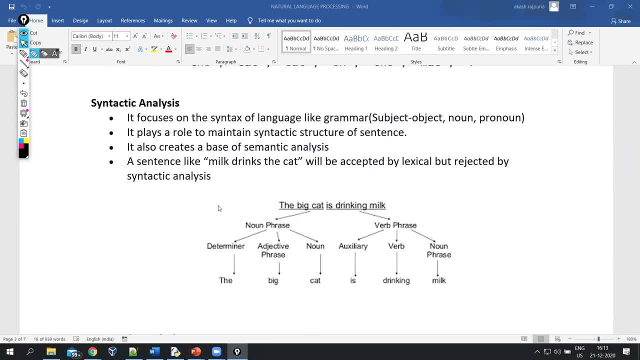 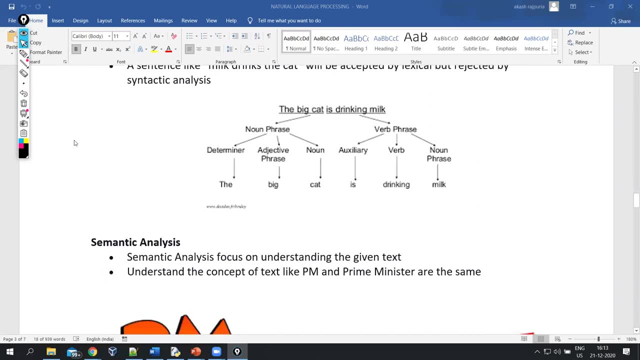 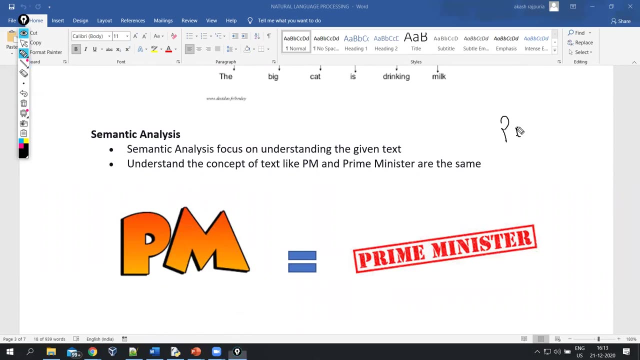 Determiner, adjective, noun, pronoun. So basically syntax of that. After that, a high level of this is semantic analysis. So now, if you are working on some complete document And you have written somewhere prime minister, In the first paragraph you have written a complete word like prime minister. 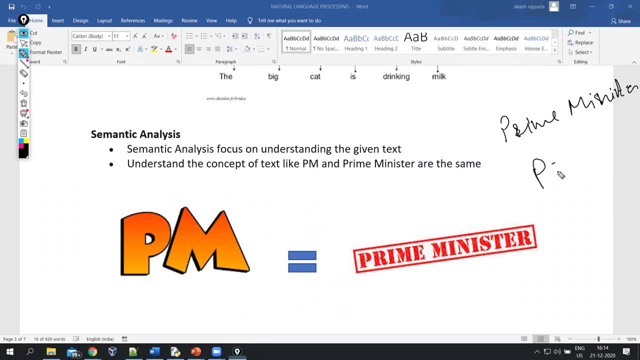 And in next paragraph, if you write PM, So your text should be able to make a right guess that this PM refers to this prime minister. It should not misinterpret that as 10 PM. So that is the beauty of semantic analysis: It understand the text. 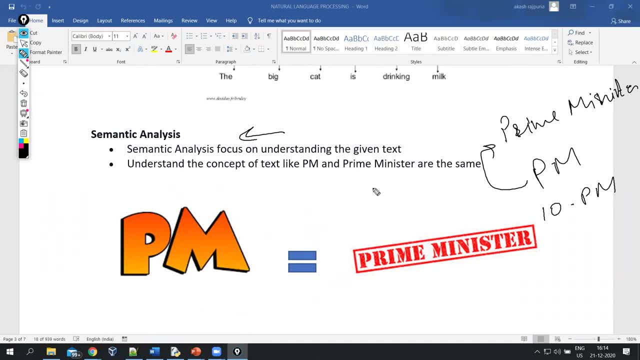 Like: what words are following the prime minister and all other things After that. it understand that PM refers to prime minister and not to 10 PM. Okay, So like you can also understand 10 PM and prime minister difference, Same way a machine can also understand this. 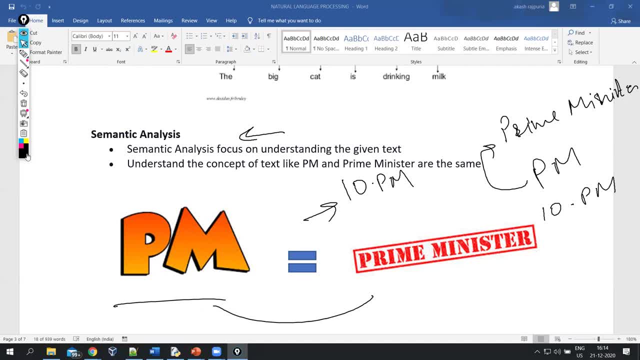 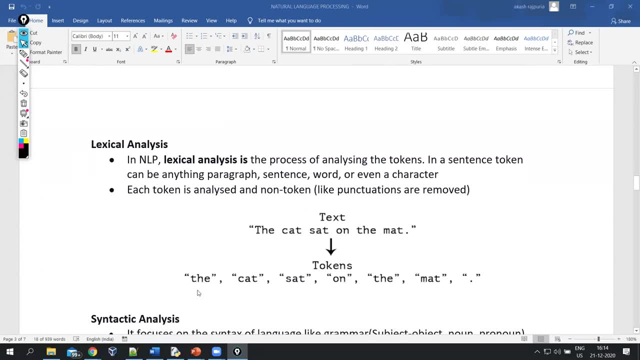 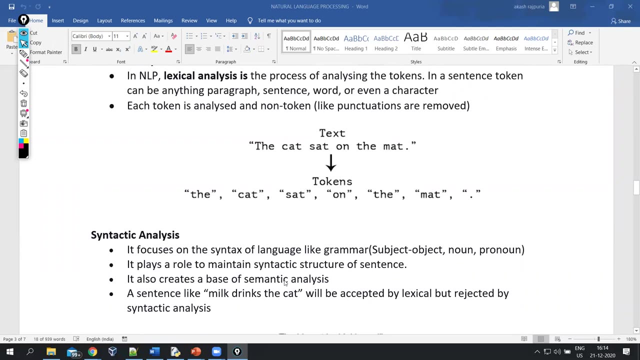 So I hope everyone. So these are the three basic things, Starting from tokenization, or you can call this as lexical analysis- Only working on tokens like the simple words. Then syntactic, more over. next step to lexical analysis. It focus on syntax. 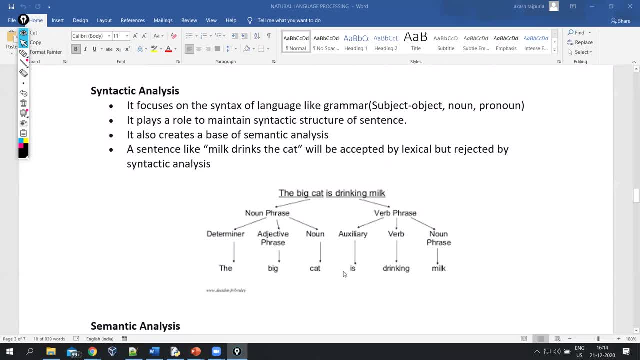 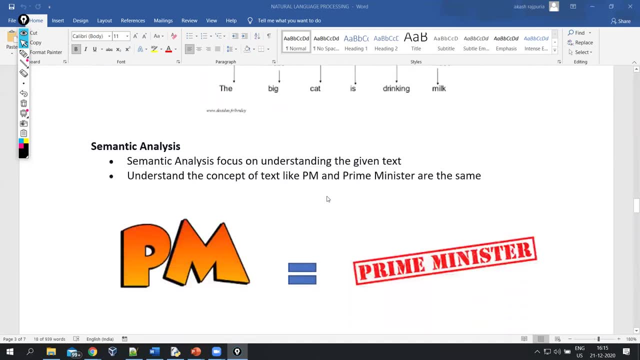 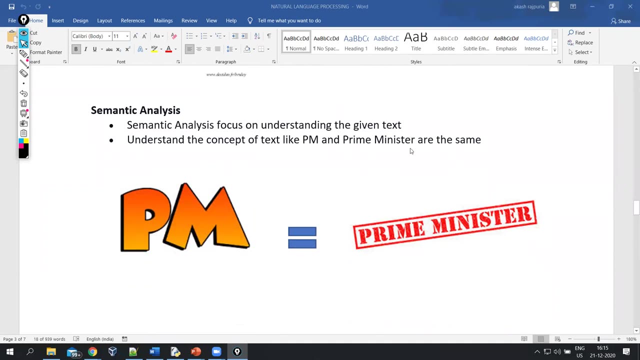 Like after. it should be in proper format, Like the bit cat is drinking milk And not should be something like milk drinks the cat. After that semantic understands the meaning of the words And interpret it rightly. Something like this: Okay, So prime minister and PM are same. 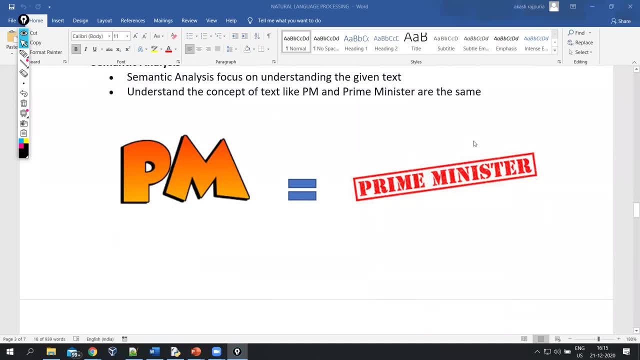 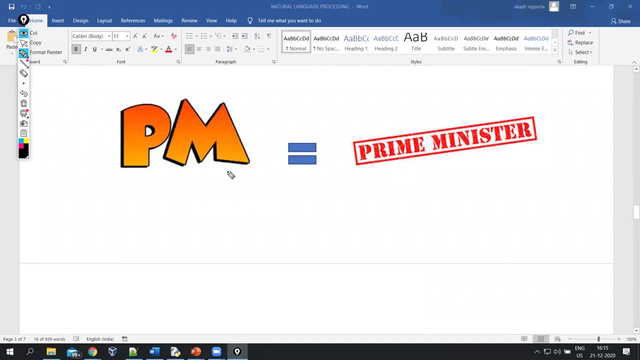 So this was the basic intuition of what text analytics is all about. In this, what we are going to do is I will explain you the problem statement now. So, for example, you have gone to a restaurant And in that restaurant you have liked the food very much. 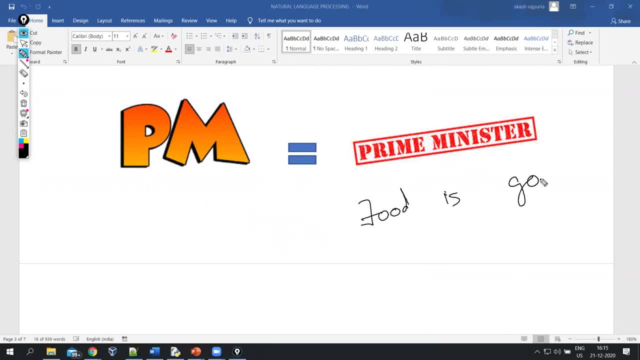 So you have written a review. Food is good, But you have went with one more of your friend And he didn't like your food And he has written something like: Food is good, Food is bad And service is slow. In this way, he has written a complete review. 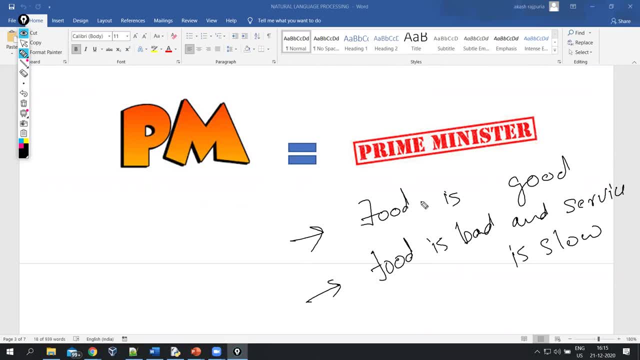 And you have also written a review. So now, being a human, you can understand this is a positive review And this is a negative review. But to make machine understand, we are doing this analysis, So if two or three reviews are there, you can read it and get that. 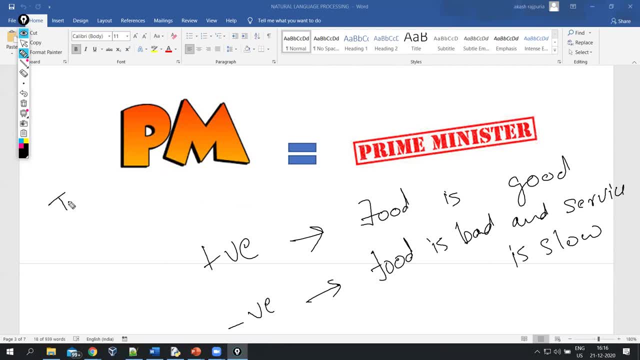 But understand if there is a big restaurant, like a Taj hotel, And there are multiple, like millions, of customers And you need to understand each one of the review, So that cannot be possible by human. So you can use machine for that Simple: you will dump your reviews to the machine. 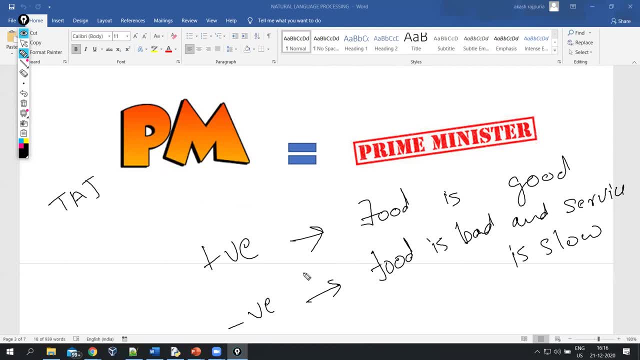 And it will give you whether it is a positive or not. So that is all about this. So we will take a real world data set And I will show you that. So, but before going that what I said is bag of word model. 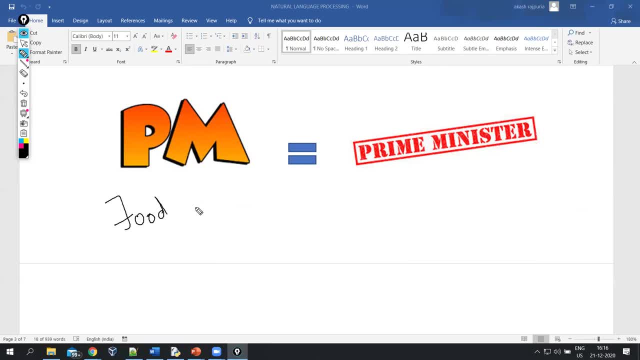 So machine cannot understand the text. Simple In simple language: food is good. Whatever text you write, machine cannot understand this. This is human readable but not machine readable. We need to convert this text into numbers. Machine only understand the numbers, like this: 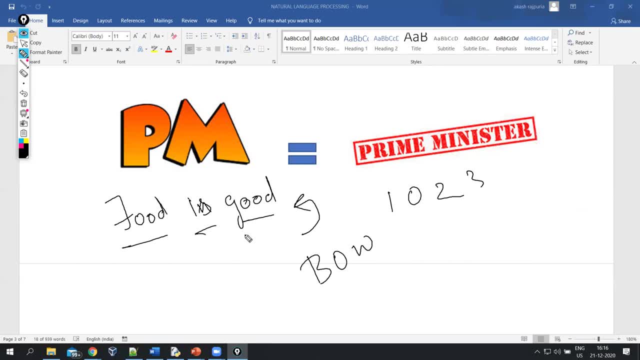 So for that, we are using a bag of words model Which will convert this string or text into numbers. Simple as that. In short, I have given you a definition of why we are using bag of word models. Okay, This is the first step towards the NLP. 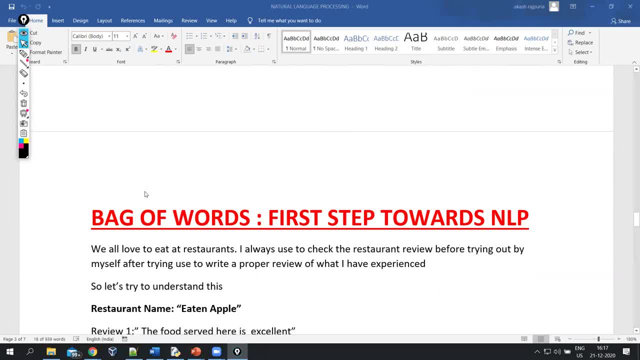 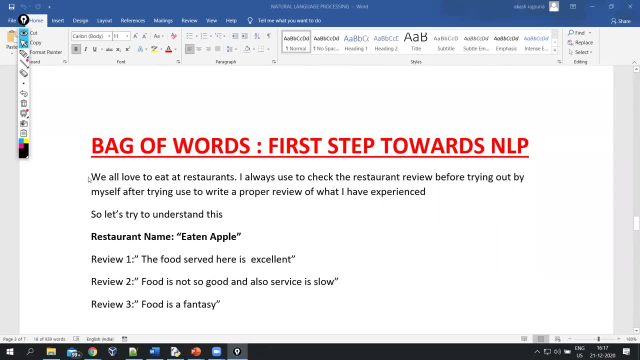 Is this part clear to everyone up till now? Okay, Now coming to our model. Like I said, this is our problem statement. We all love to eat at restaurant. I always used to check the restaurant review before trying out myself. So you can get the reviews- one, two or three- like this: 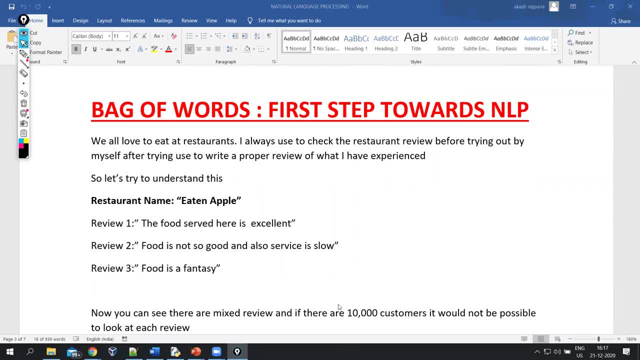 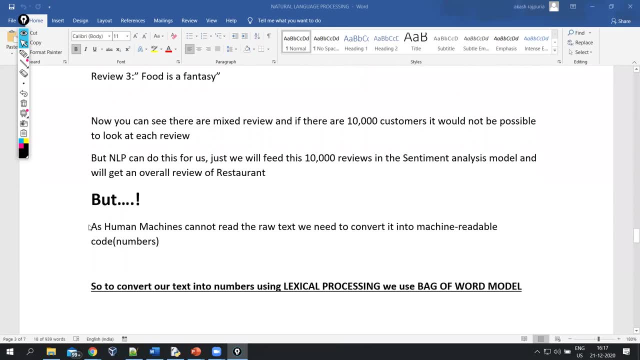 But if there are 10,000 or more customers, It would be not possible to look at each of the review. Okay, So for that we are going to use bag of words model. So, as machine cannot read the raw text, It needs to be converted into machine readable. 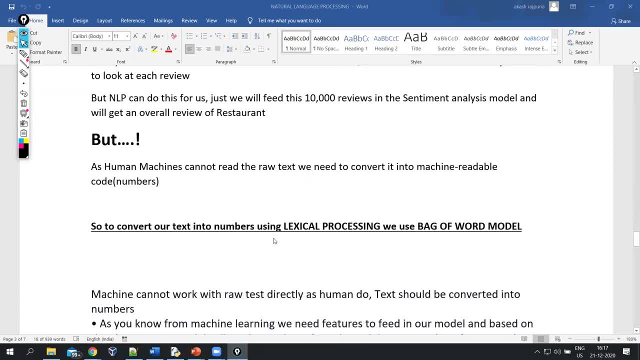 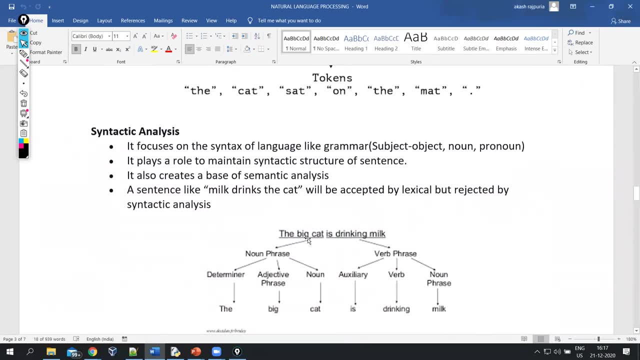 That is numbers. So to convert our text into numbers, You will, we will use lexical processing. So, like I explained you, We will use a simple first part, that is, lexical processing here, And this one lexical analysis. that is token one, This part. 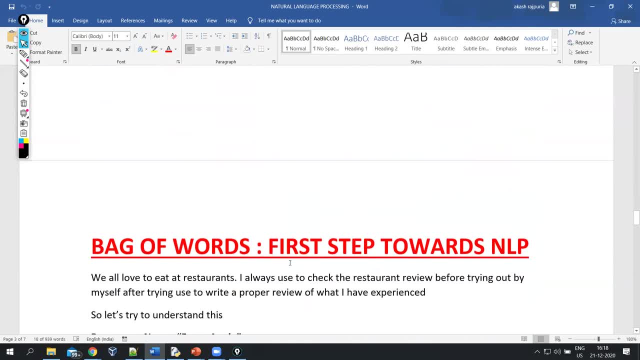 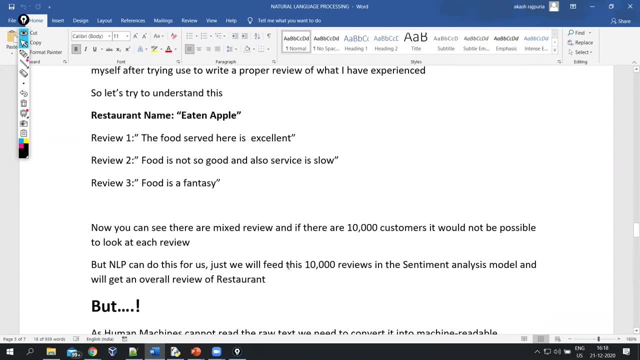 And we will see how a more machine can understand your text very good, in a very good fashion. So for that we will use bag of word model. So I will explain you how it works. So what bag of word model do is. I'm explaining you the theory behind the algorithm. 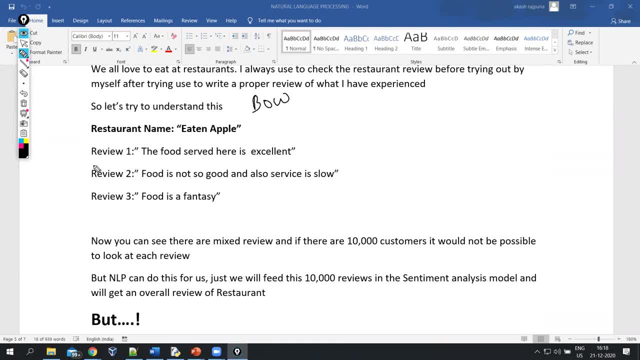 So bag of word model is an algorithm. So now what it will do? it will take all your reviews. So this is review one, review two and review three. It will calculate. first step is to get the unique words. Okay, First is unique words. 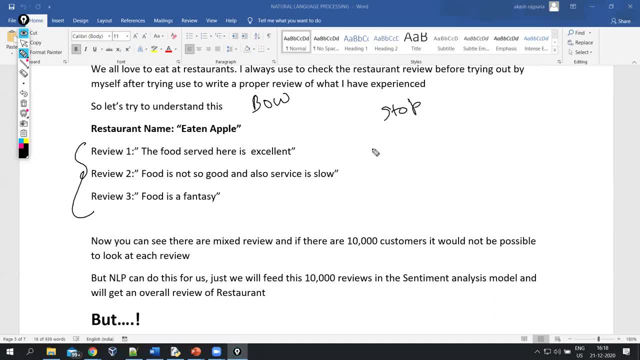 So, before that, I will explain you what is stop words. stop words are something which are, moreover, in every sentence, but are not much useful for the sentiment. like the words is the is, so also is is so these are all the kinds of stop words which are not much useful. 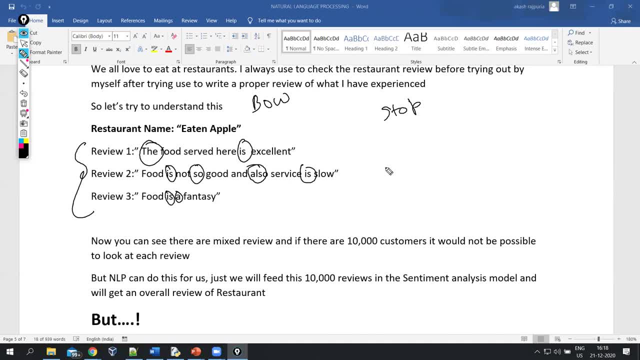 in the sentiment analysis. So I will explain. I will give you one library which gets this stop words and removes all the stop words and remove that. so basically, while understanding this sentiment, we will remove this stop words. as simple as that. So, all after removing the stop words. how bag of word model works. 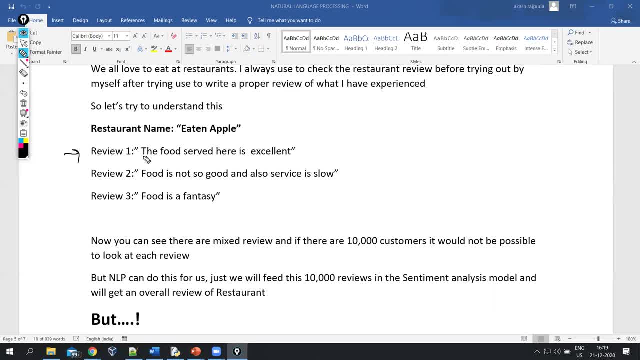 So what we can do is we have first review, so we will count the unique words. for example, the unique words are: the food served here is excellent. Okay, These are the different words. for example, And we have next sentence as well, in that food is already there. 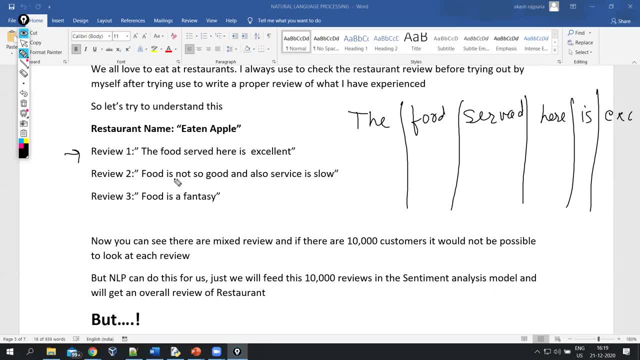 So we will not write that food again. then is so: is also there not? is not there? So I would, for example, right here: not sorry, I am not here space, So I would write here, so you can write it anywhere. not in this way, you can write it. 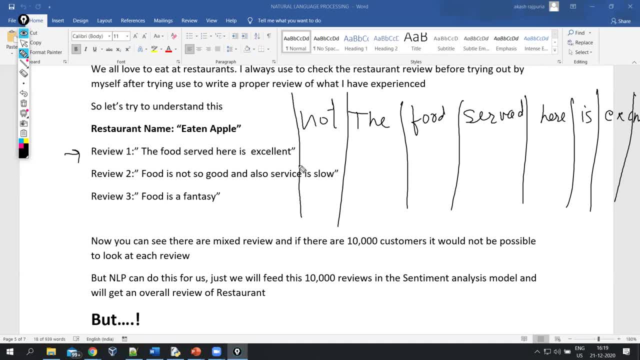 now I will check each and every. so in this way we will create all the words in the column. Now we will check whether that word is appeared in the document or not, For example. I will remove this, not for you. You can understand from this now. 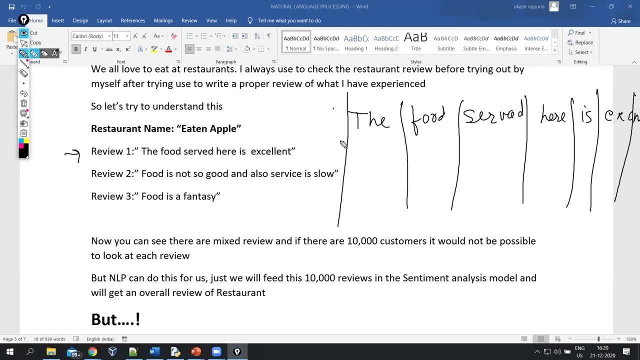 So this is my matrix, where I have document one here, document two and document three. So in this way I have created three documents now. So now in first document I will check, the is available. Yes, So I will give one here. The food is there. 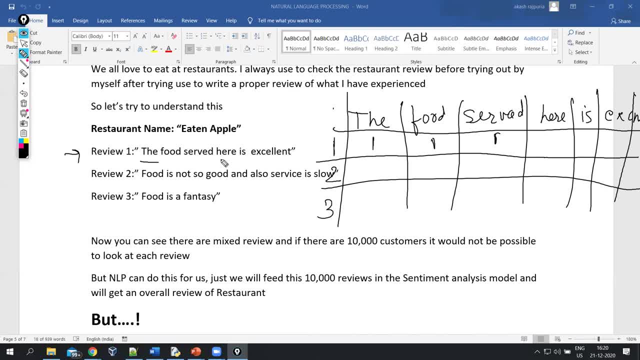 Yes, Served. is there? Yes, One? Okay, If it has a here. is there one is. is there, Yes, Excellent. is there? Yes, Not. is not there. So last is for not, So I will give zero here. 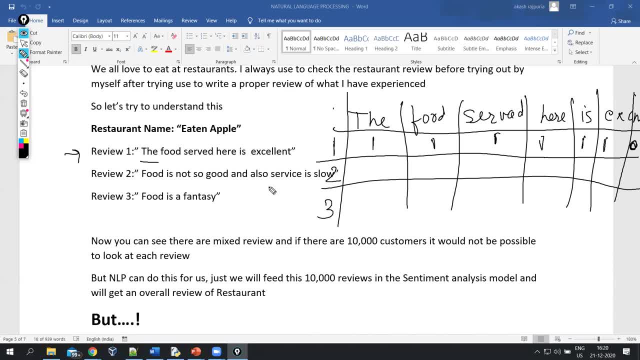 Same way. food is there in the second, though is there in the complete sentence. There is no, though, in the second review. Okay, Now focus on the second review. There is not there, So zero would be there. Food is present there, Yes. 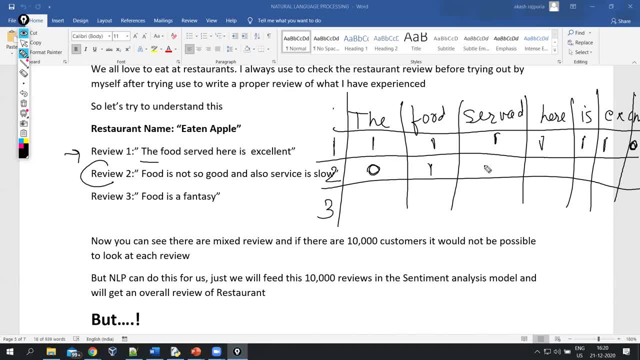 Served is there. No, Service is there, but not served. So we will give zero here Then not. ease is present there, So I would write ease and one here. So if the ease appear two times, I would write here too. Okay. 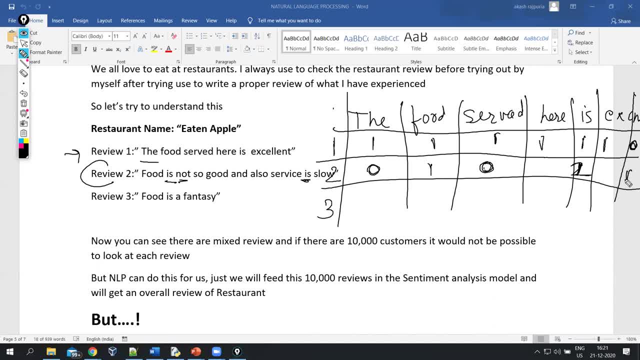 Simple as that. Now, same way not, is there? So I would write one here. In this way, I will fill this complete matrix and what I get is my numbers. So this numbers are, for example, one, one, one, one, one, one, one, zero. This for first statement. 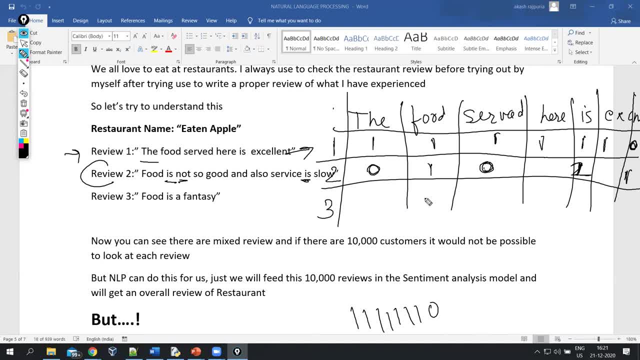 For second statement: I have this way. So in this way I just count the unique words. So, as I said, we can remove the stop words. So we will remove this, the here ease. Okay, In this way we will remove And we will have this type of features with us. 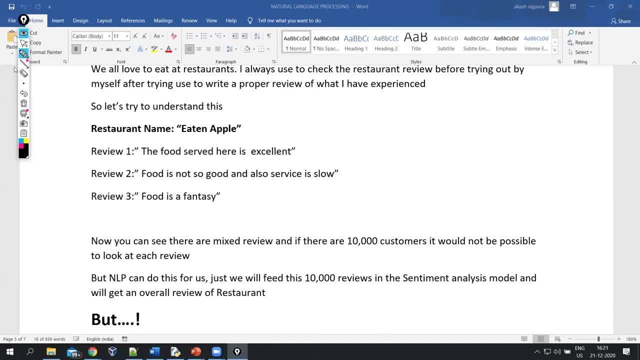 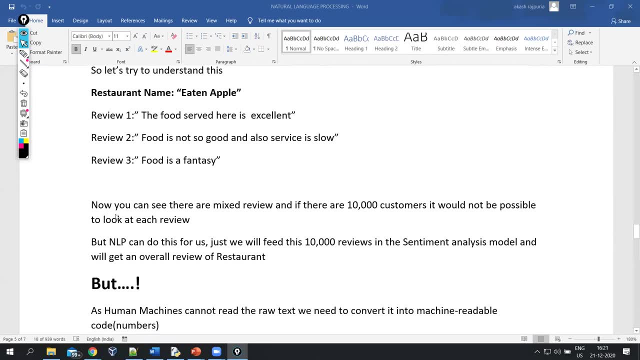 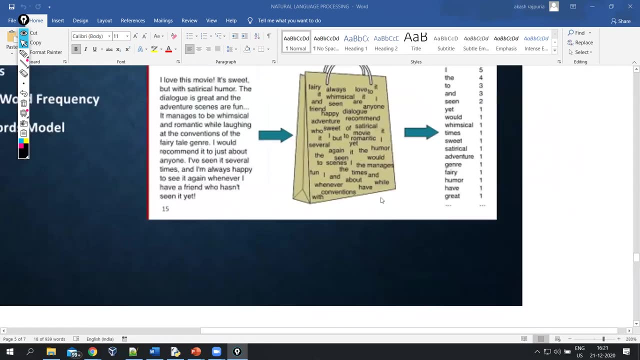 Okay. So this is simple, called as bag of words model, where you first count the unique words and how many times it has appeared in the document. Just that, nothing else. Okay. So this image would make it more clear for you. Like, I have this complete paragraph. 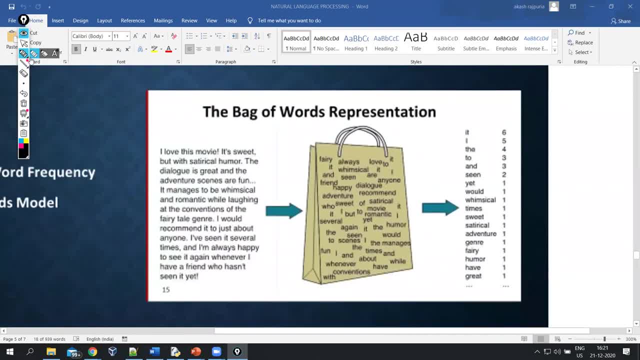 So, as you see, I have taken it, tokenize it So in the lexical way, like each and every token I have gathered here, And after that I have converted a list of all the unique words, something like this, Okay, And counted it just how many times it has appeared. 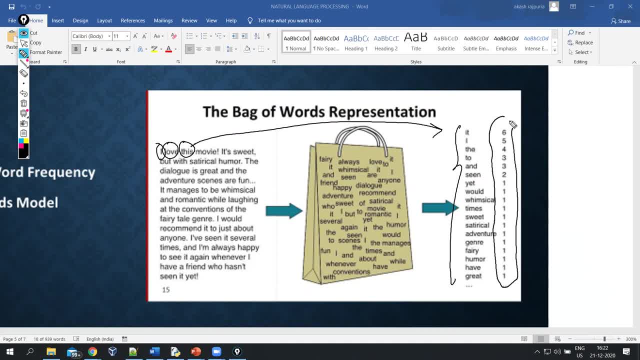 So this is my complete text now and I can feed that number to the machine to understand whether this text is positive or negative. Okay, So I will give you one interesting fact about this. It is called bag of words model because, as the things are in the bags are random here. 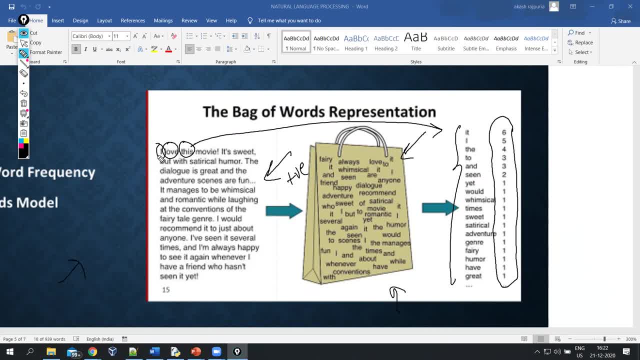 the words are also random, So it doesn't focus about whether the eyes appeared first time here or here it has appeared. it will just put into the bag randomly So you can see all the words are random here. That is why it is called as bag of words representation. 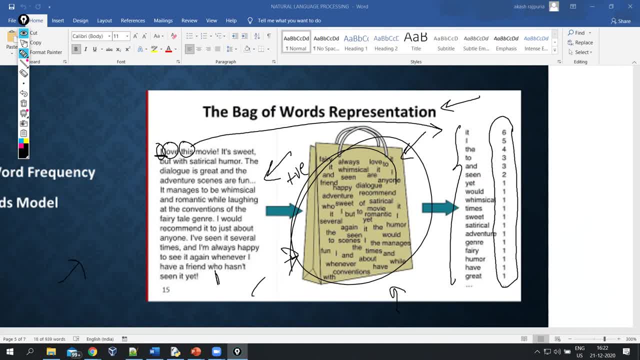 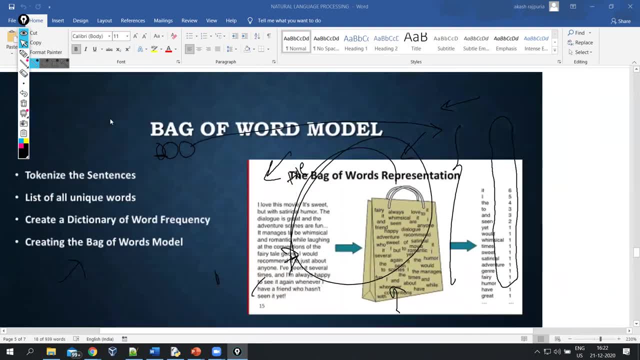 So your text is the represent into numbers using bag of words. I hope up till now everyone is clear. more part would be clear when I will show you the coding section of this. but this is all about bag of words model, So without going first away, 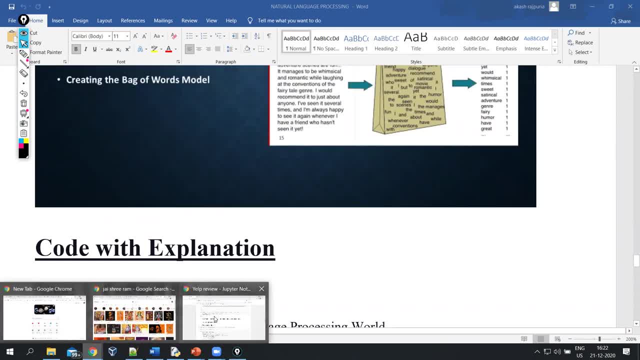 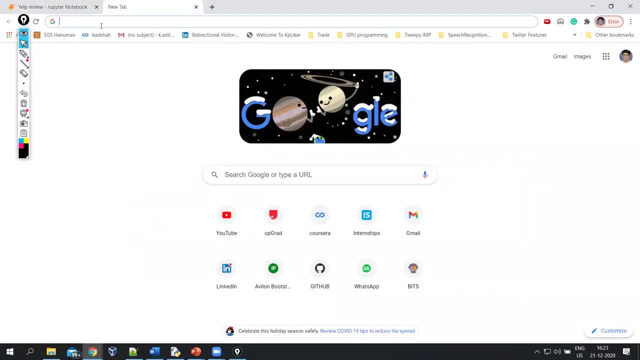 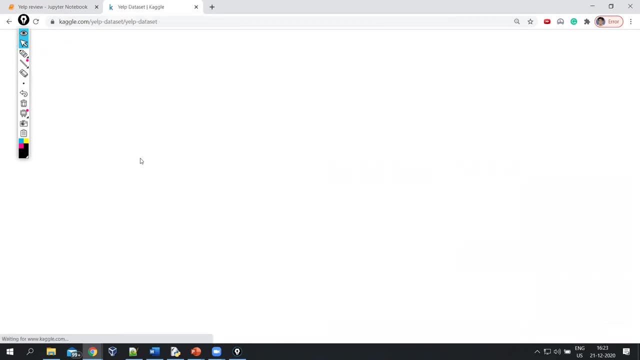 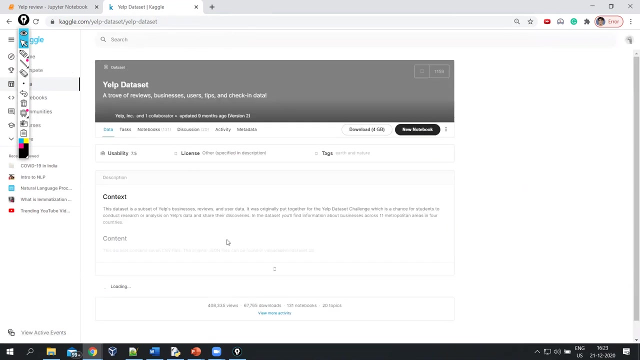 I will explain you the complete case study now. like yes, so I will. you can download the data set from here like Yelp Kaggle data set. Okay, So this is a restaurant review data set where we have multiple restaurants and approximately 10,000 reviews. we have and you can download this data from here. 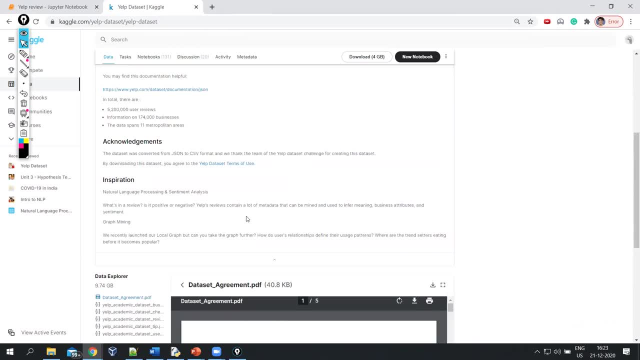 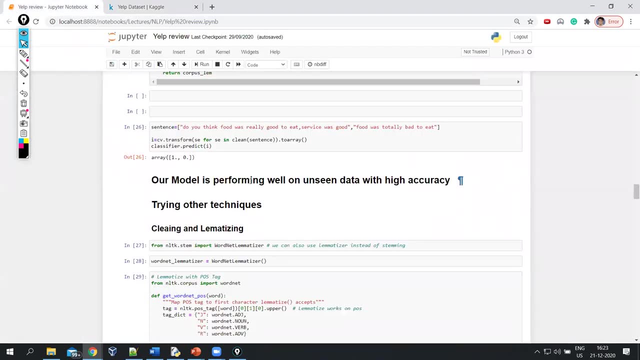 This data set has 10,000 more more reviews. It has many reviews with you. You can download it and work with it. So I will explain you the code now. First of all, how it works so simple. first We will have this libraries to remove the stop words. 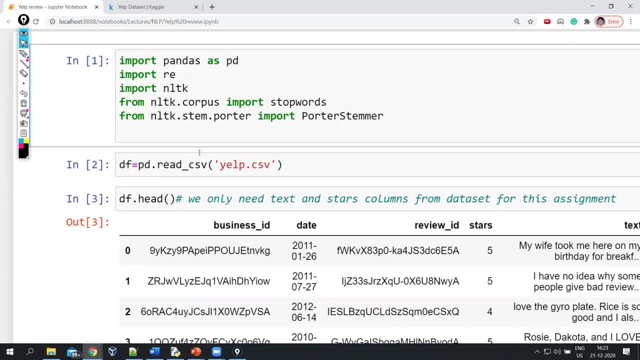 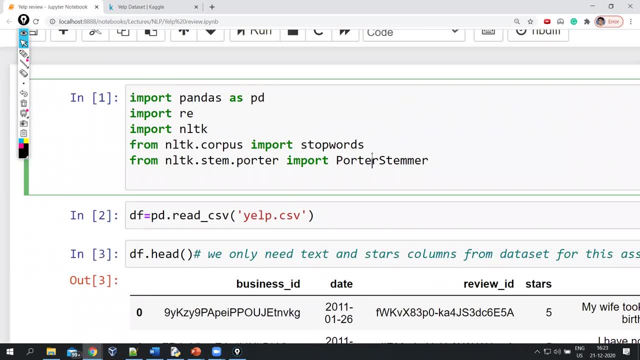 We have this library. I will explain you. one more concept in this is that is called a stigmatization. Okay, why it is used. I will explain you that as well. So this is the complete code of getting the libraries. only this. libraries are needed like 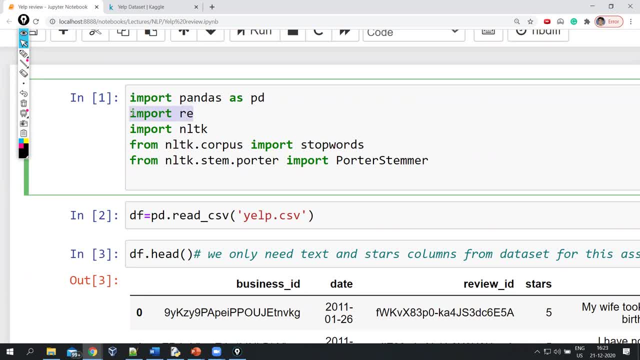 this: This is re library. that is regular expression to remove the punctuation. So this library is used to remove punctuation. This is pandas library. Then NLTK is used for this top words and the stigmatization. So everything is available for you. 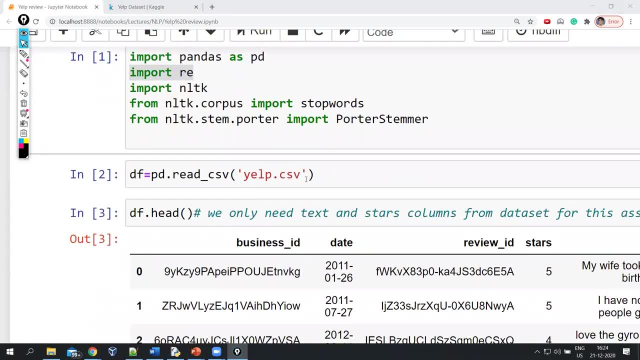 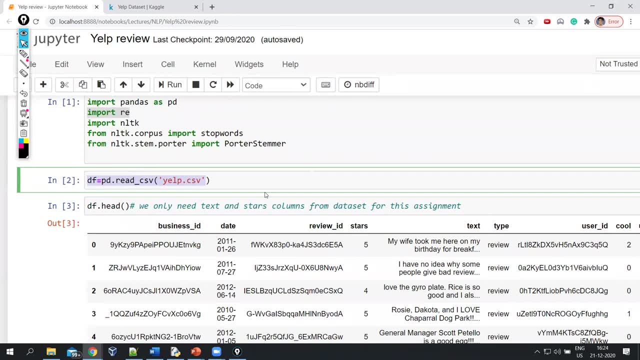 I just need to understand how it works. So now this is my CSV file. You can see a head portion of it, like the five top rows. using this head function, You can see that. sorry, Yes, using the head function You can see that we have different business idea, business ID, date, review ID. 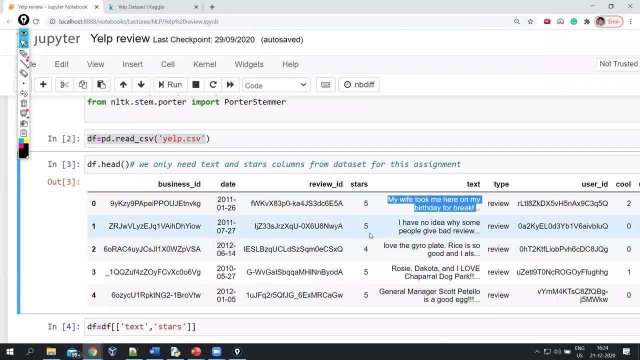 This is my text which I need to analyze. Okay, and this are my. some of the stars are given like you give star 1, 2, 3, 4.. So in this data set I have star from 1, 2, 3, 4 and 5. 1 means bad review and 5 means good. 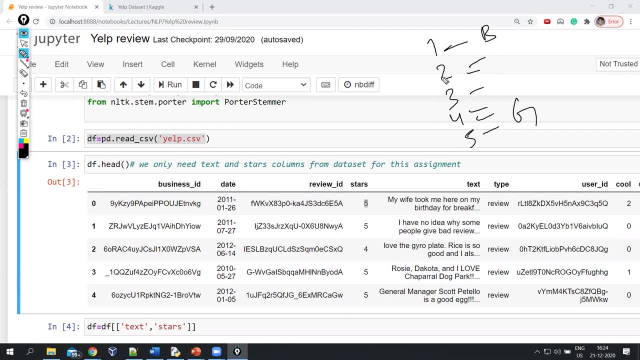 review. So in this way, these are the some things to start. You know all about this, How Amazon works. same way Yelp also works. Now, after this, I have many other columns, but for this the, as this is a very basic understanding of how it is. 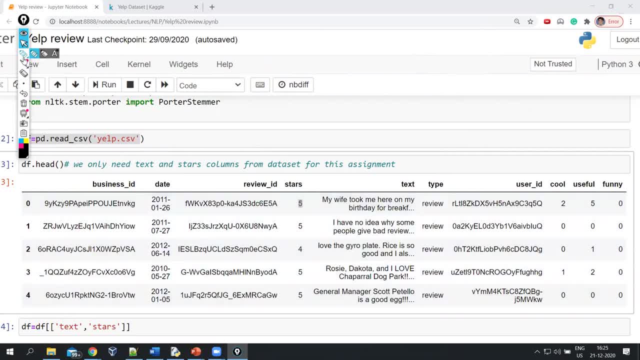 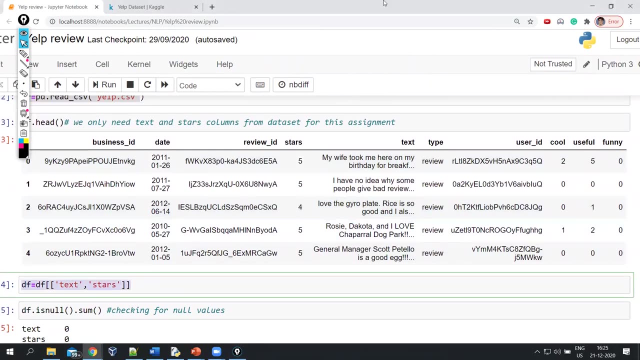 So I will explain you, or we will only work on two columns here. that is, first is this text column and second is the stars, all the columns we will remove else other than this. Okay, coming to the part, for that, I have written this code to extract only the stars from it. 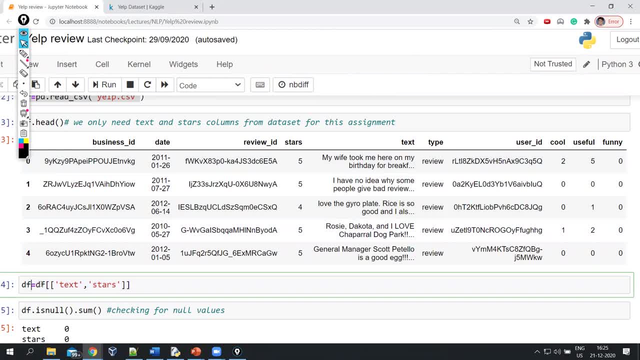 only the stars And the text part. So this is DF, the data frame name, and in that you need to give a list of columns. So if you have only one column you don't need to give this multiple list. But as I have two columns to extract, I will use this text and stars. 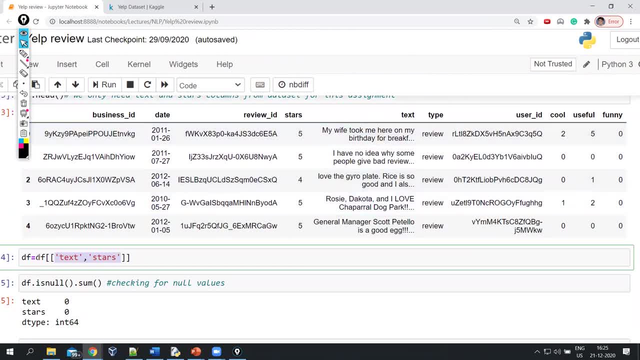 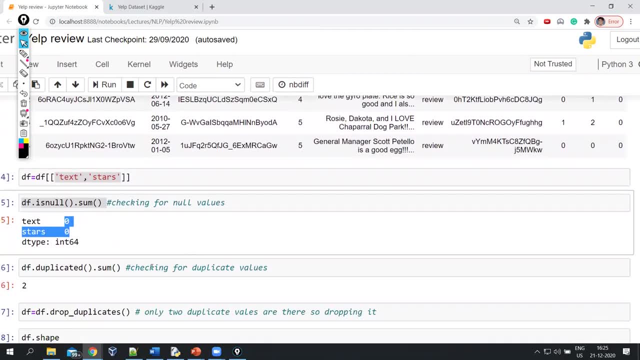 So I have my only text and stars. I explained you. I will check whether it is null. So I'm checking for null values. There are no null values in this. I will check if there are duplicate values. Okay, so I have two duplicated values here. 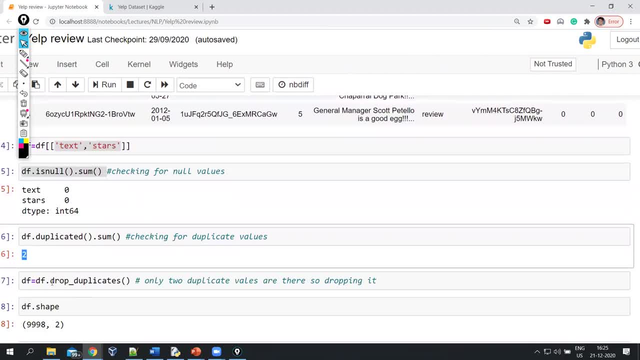 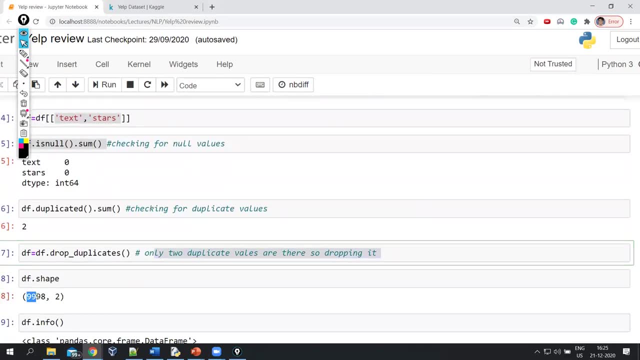 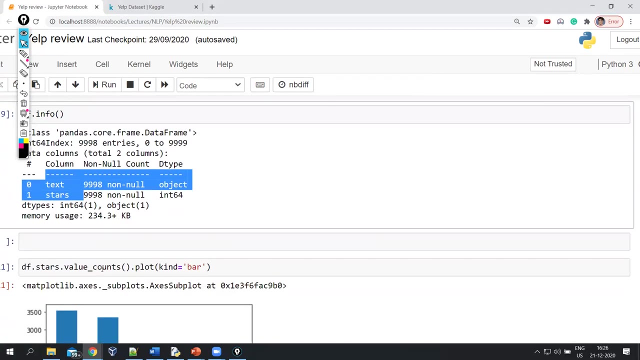 So, basically, as the count is very less, I will drop the duplicates using drop duplicate function. So only two duplicates there are. therefore I am removing it. so you can see the shape now that is 9998 rows and two columns. so you can see that as well. after that I will plot. 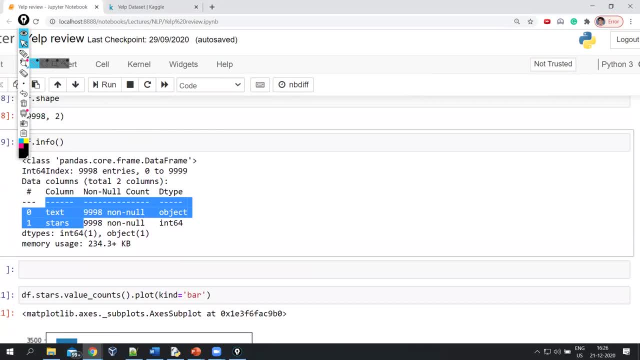 what I have done is I have plotted how many. so I have stars in this way, like one, two, three, four and five I want to see. so each one of this is my class. So what? in this exercise, what I am going to do is for first class. 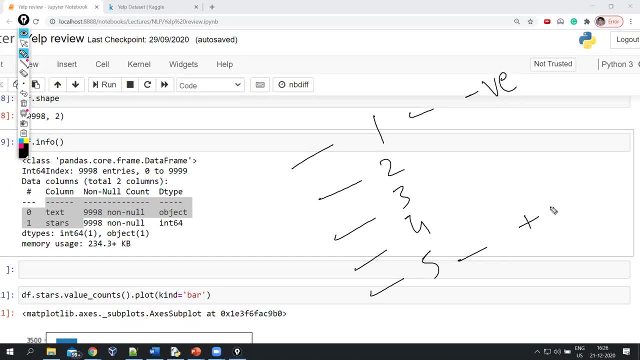 I am saying that it is a negative review for five class. I am saying it is a positive review. all of the stars I am going to drop off. Okay, to make it very simple to understand how back of word model works. Okay, coming to the section you can see the star counts. 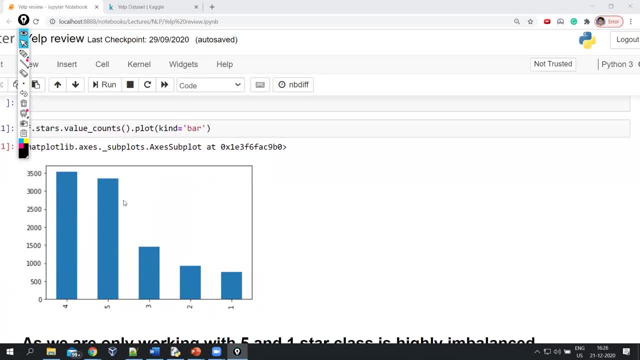 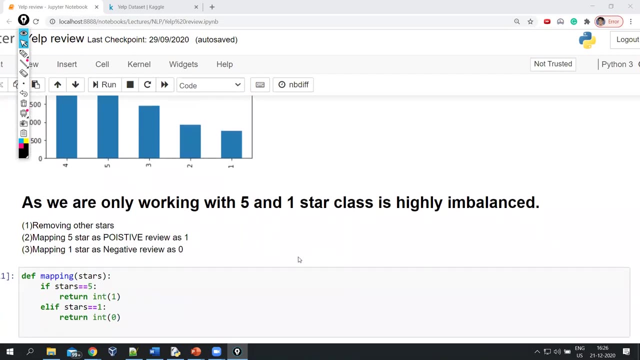 So four star has the highest. people has given four star maximum, five star a little less and one star are very less. So this is a highly imbalanced data class, But the focus, The focus here would be to understand back of words model. Okay, so, as we are working on fives and one star class is highly imbalanced. 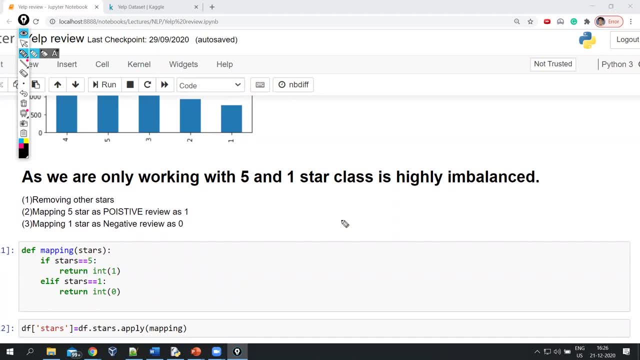 So I am. what I am doing here is yes, So I am explaining you the part. now I am removing the stars. So, like I said, one, two, three, four and five stars I have. so I am removing this to, I am removing this three and four. for that I have created this function, which will take the 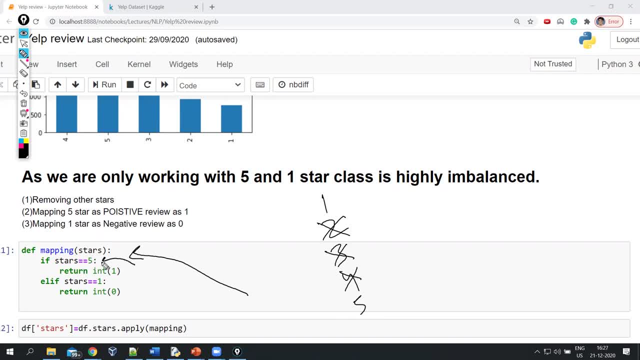 stars column. So I have the stars column. It will check whether the column is five, If the star is equals to five. if it is five, it will return one. Okay, so one means the positive review. for positive, I have coded this as one. 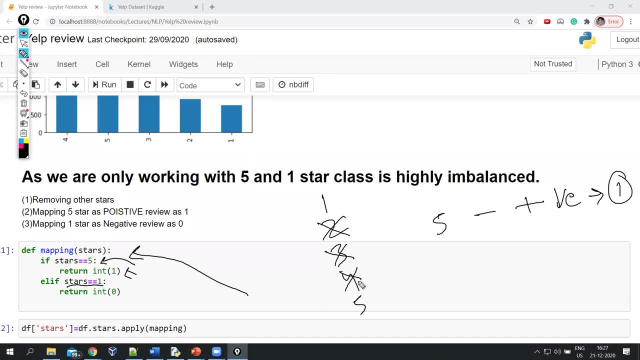 If my stars is equals to one, Okay, it will see. if the stars is one, it will code it as negative review, which means that zero it will return. So in this way, what I have done is I have a stars column here in this. I have stars as. 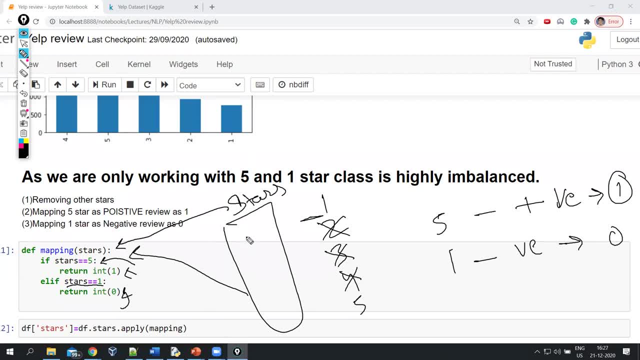 named stars, So I will pass the stars to this function and in the stars, for our example, I have one, two, five, two in this way. So it will check for one. one is there, So it will go into the section, else if part, it will return zero here. 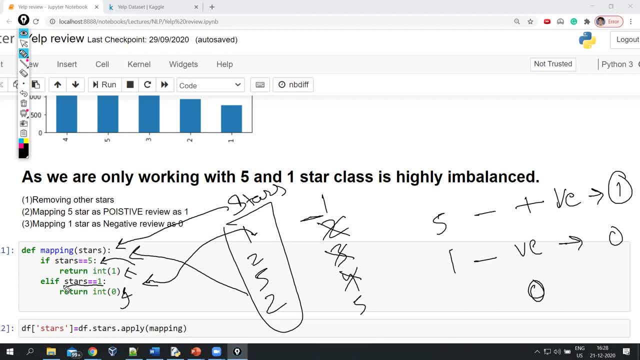 So I would get zero. now, two is there, So two is not in the statement. So it will return a nan value. Okay, because two is not there anywhere. So it will give you a nan value after that for five, it will check. I will got one here. 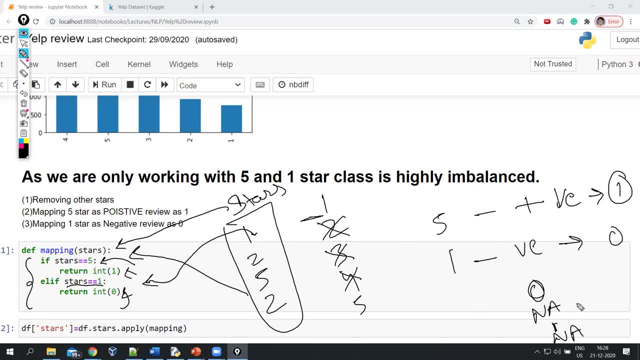 same way for two nan values. So I am just removing the nan values at the end and I am remaining with zeros and ones. So zero means negative review and one means positive review. Okay, so I have coded everything, I have applied this star to this and you can just part df. 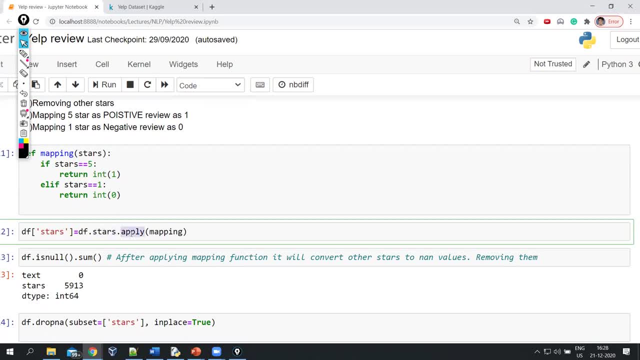 dot. column name: dot- apply. Okay, this is the function and you just need to pass to your defined function So it will go. every stars value would go into this, check it and return that. So after applying, you can see the null value. So this menu are the null values. like I said you, for remaining star, it will create null. 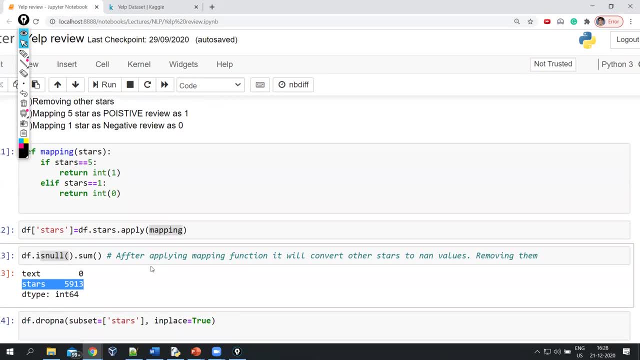 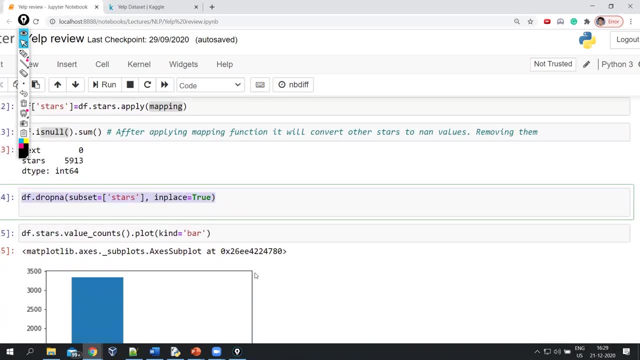 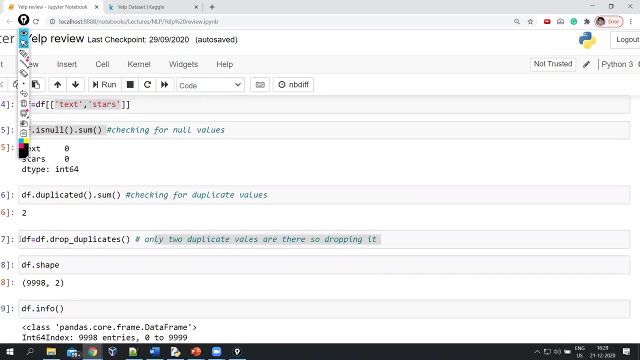 values. So 5913 are the null values. So I will drop that null value simply using drop any function and in place equals to true, is you don't need to again assign it. Okay, like I have assigned here again to df, like this df, if I used in place here, I just 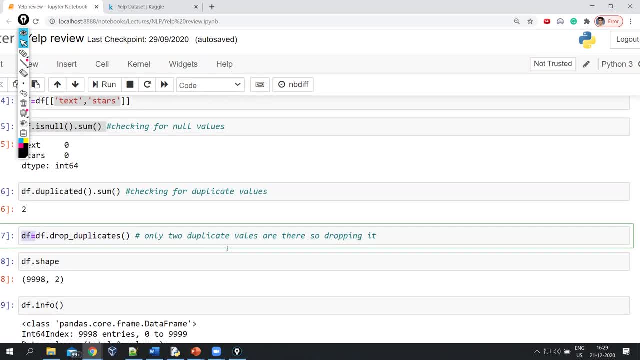 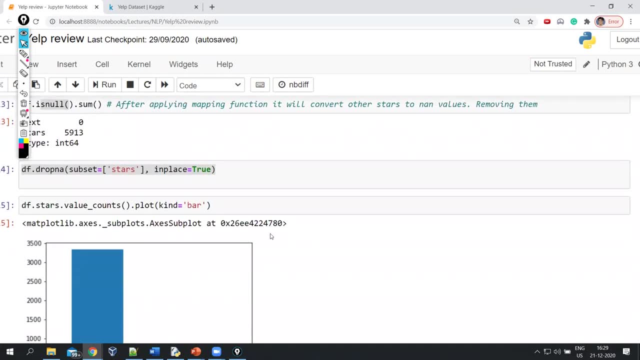 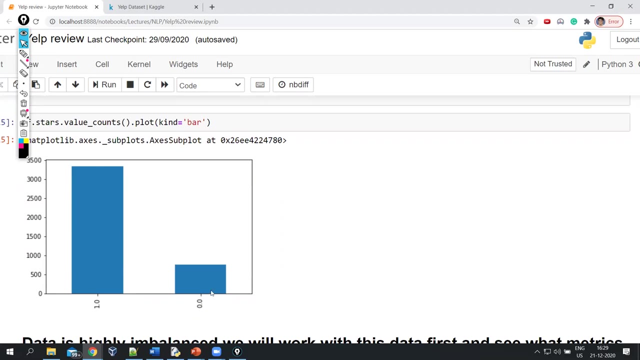 need I can remove this highlighted part. So in place equals to true is make the changes there and their self in the data frame Simple. Okay, after that I have seen how my class looks. so one class is highly, which means I have more number of positive review than the negative reviews. 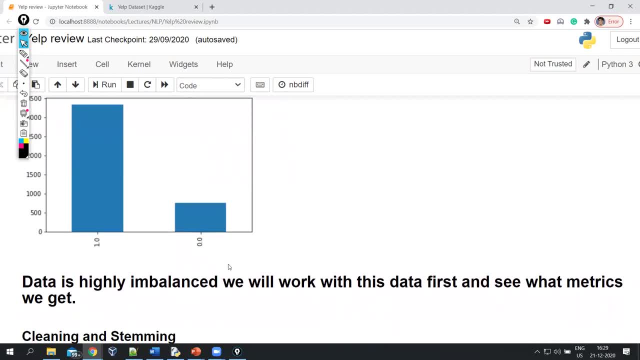 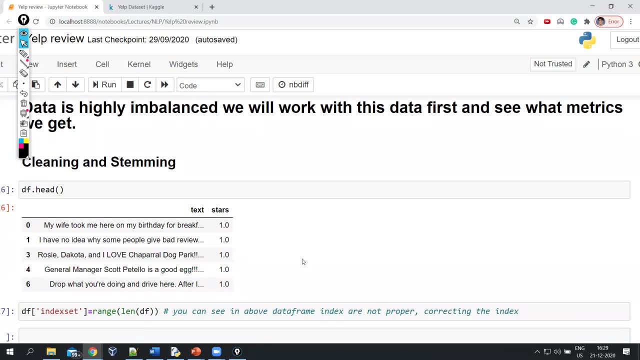 So this is basic data. cleaning has been done. Our data is highly imbalanced, but we will start with working with it, Okay, Okay. before going to this, I will explain you what is stigmatizing, So stigmatizing, Okay. So stigmatizing is also very simple. 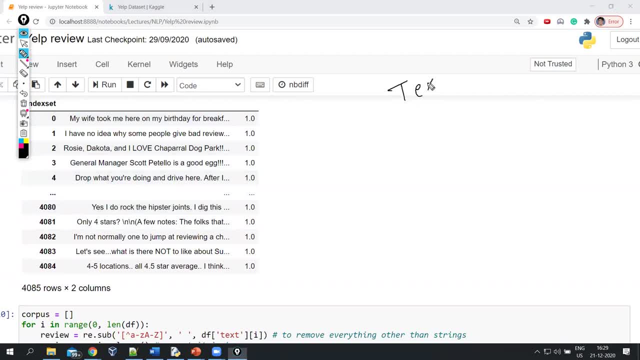 Like, for example, you are working with a text data. now in text data you have a word eating. Someone has written a review and he has written eating there- I know some was some was the sentence- and it has a word eating. Some of your friend has also written a text and it has a word eat. 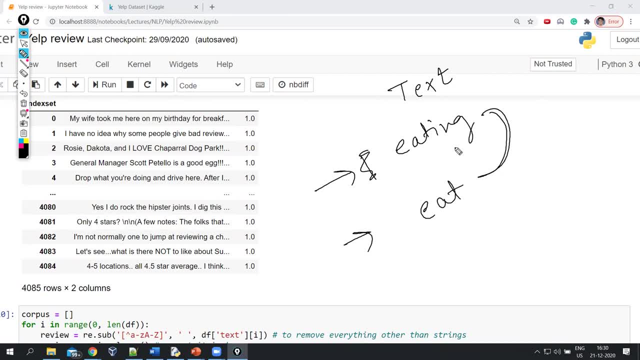 Okay. So, as you know, this two words are similar but due to this ing, it will create another column. So, like I explained you, Every word has a unique column. So eating would also create a one column, and eat also would create a one column. 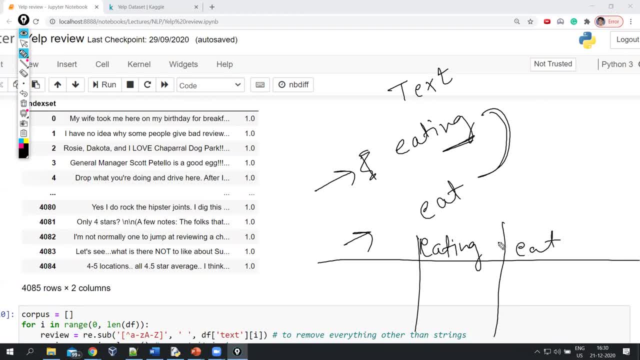 So this is extra feature. This is redundant. features are added, So what we will do is stemming is simply chopping of the last suffix, like ing is removed. Okay, so same way for every words are there. It will just remove the ing and the suffix part. 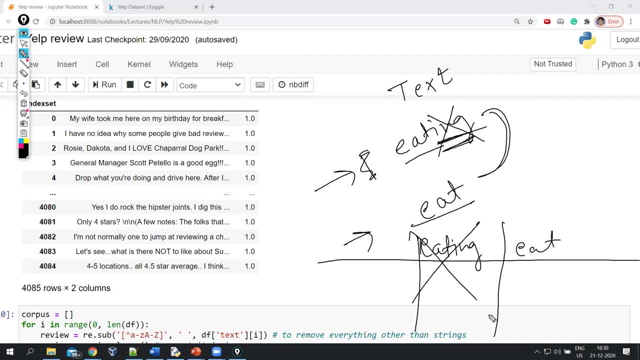 So you will get eat and eat now. So it will not create this another column. Only one column would be there. So it will check the, it will take the text, it will remove this ing part and then it will return you the word eat. 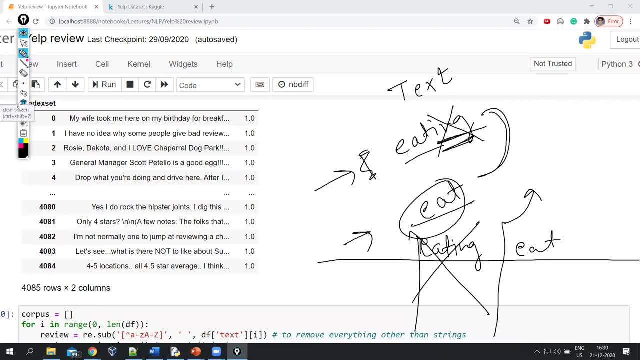 Okay, So this is a simple thing about stigmatizing. So stigmatizing is used to remove the ing part. Okay, One more thing to understand while working with text is, so you can understand that word people and this people. Okay, so this, here P is capital and here P small. 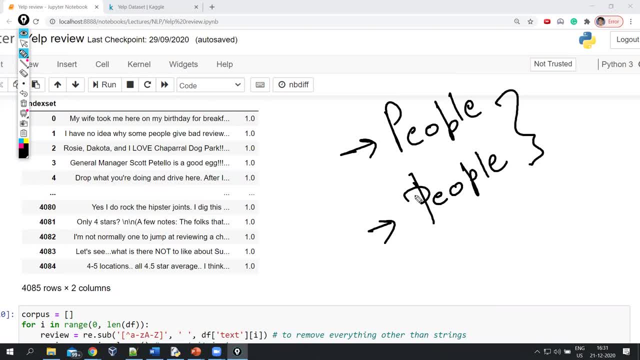 So this two are similar for a human, but for machine they are different because there are ski, codes are different. So this is case sensitive now to make. also, what happened is if you give this type of text to computer, it will create another column for people and another column for this people. 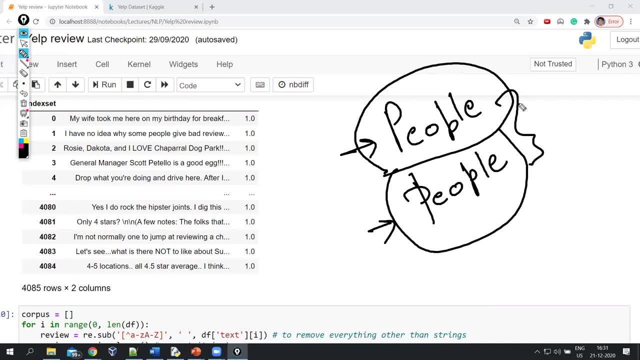 So you will have again redundant features. so you can convert all of them to uppercase or you can convert all of them to lowercase. simple formula or simple logic. Okay, So I have done all this for you, Like, first thing that, like I said, I will remove the punctuations. so punctuations like 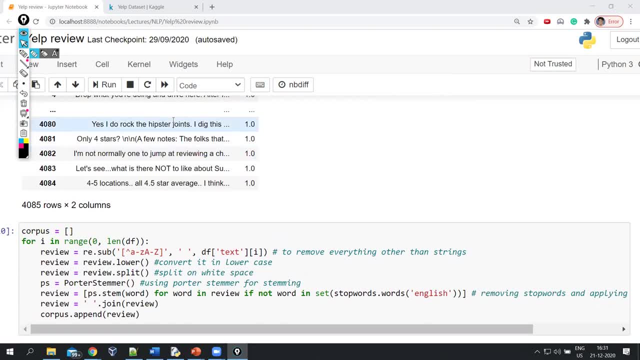 this question. mark the slash and this bracket. Okay, this digits. I will remove the digits as well. this dots, this dots, So it all be removed. for that I am using a library that is regular expression. This is very powerful library. This is the code for this library. 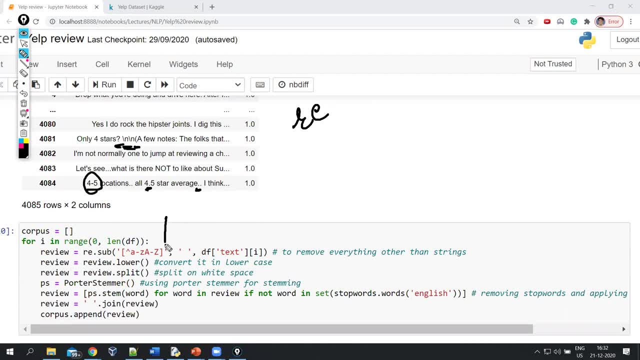 This is the code for this library. This is the code for this library Like. it states that the star is for starting to. it is for pattern matching. Now, the stars means that to check at the starting of the word Okay, And this is the range. define like the ranges from A to small, A to small Z and capital you. 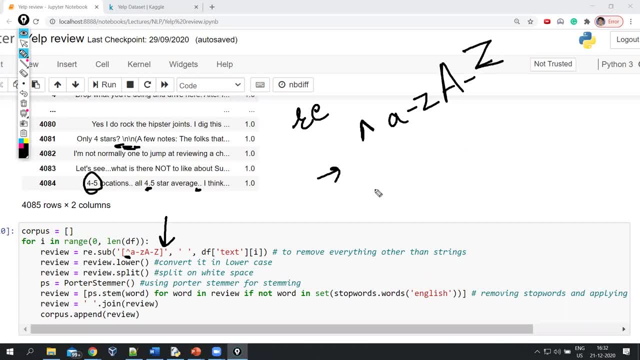 took capital Z. So it states that any word starting with a small A or small Z up to anything like small A, A, B, C, D, E up to small Z, or starting any word with capital up to capital z, you just keep that word. if the word is starting with this range, keep that else. 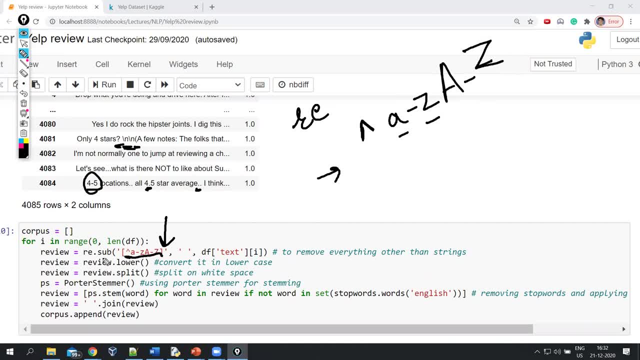 if there is something else other than this, you substitute it. so i have used a substitute function here. substitute it with a blank space, okay, so, for example, you have a review food comma. good, in this way. so it will go into the word. it will check f. it is starting with small. okay, it has. 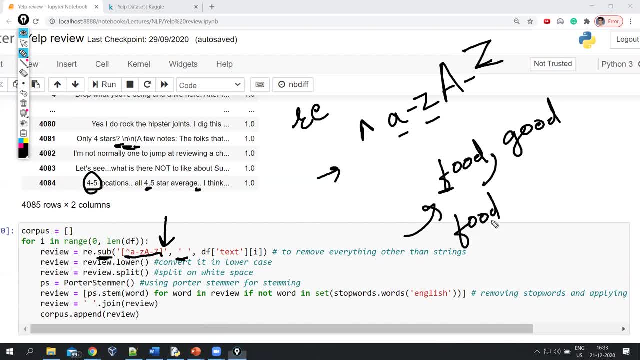 small letter. so it will keep this word, that is, food will be kept because it is analyzing each and every token, so it will keep the food word. then it will go, because it is in the range of this small a to small z. then it will check this comma. so comma is not in this range, so it will. 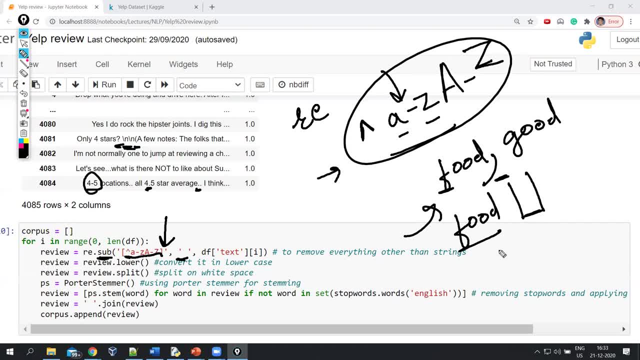 just create a blank space here. in this way, a blank space will be created. then good also start with this range. so good will also be there. so in this way it will remove all the punctuations. so this is a simple logic: to remove the punctuations, to remove everything other than strings. even the digits would also be removed. 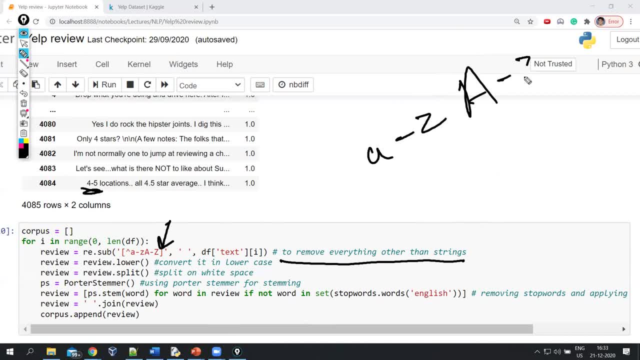 because they are not in the range of a to z and capital a to z. okay, after that i have converting everything into the lowercase using this lower function. after that i am using a split. so this split is something like, for example, you have a review food good is in this way, so it will split. 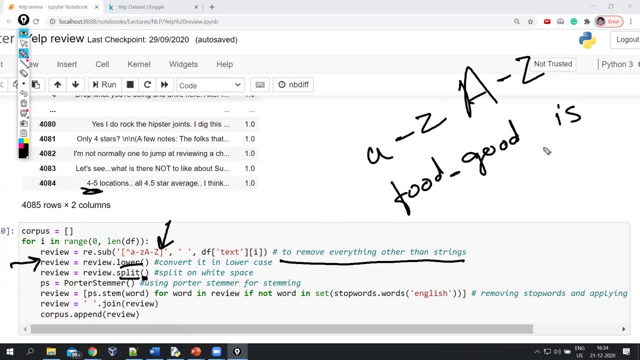 if you don't give anything in these brackets, it will split on this blank space. so this would be your token. this would be your token in this way simple, as i explained you the token part. now, i have used the spotter stemmer class here, which i have export imported before, so now this would 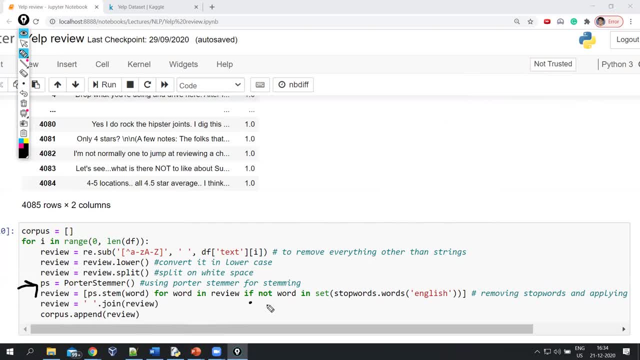 create object of it and this is something called as list comprehension. so it starts with: it will check every word in the review for word in review. it will check every word. it will take every word if the word is not in stop words. so, for example, you have a statement: food is good. 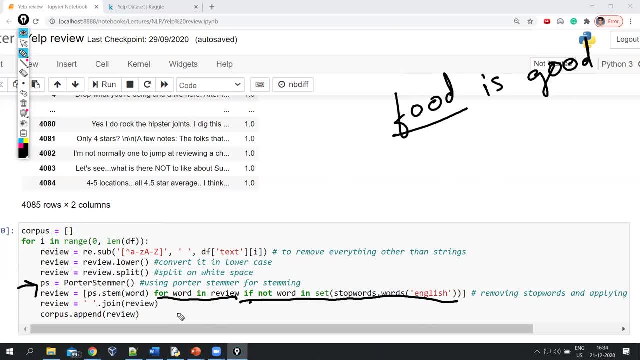 so it will take the first word that is for word. in review it will check whether a food is in stop words. so food. food is not a stop word, so it will return the stemming of the word. okay, it will do a stigmatization on top of word, so food. original form is only food, so it will return you the food. 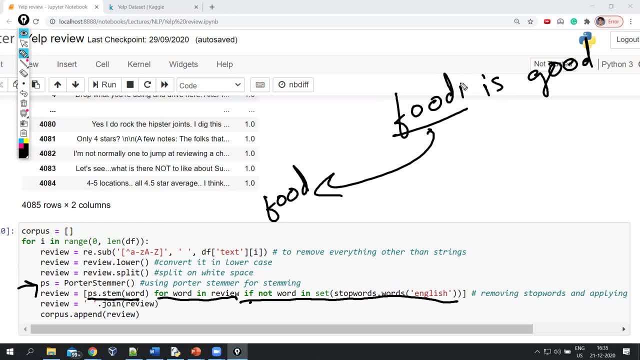 as it is okay, for example, if, instead of food, you have fooding here, for example. this is just a raw example, so it will check. it will first check whether the fooding is in stop words. no, it is not in stop words, so it will do, at the end, stigmatizing. 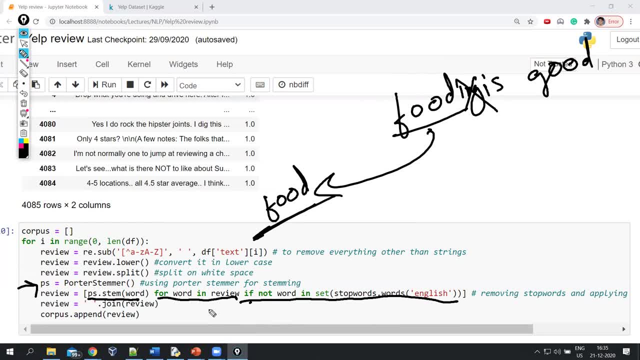 so ing would be removed and you will get food. okay, after that it will move to. next word is: now is a stop word. it is a stop word, so it will return. it will not return anything. okay, because i have written: if not in, if it is not in stop word, then only return. so it is a stop word, it will return. 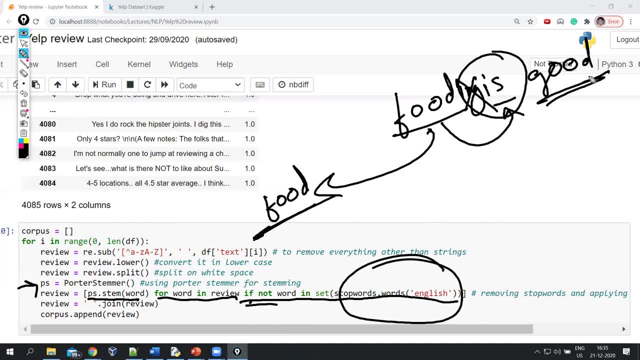 nothing after that it will go into good. so good is also not a stop word. it will again go to stigmatization. it will. it will do a stigmatizing, like it is a original word, so it will do nothing on it. so you will get a new sentence as food good instead of fooding is good. 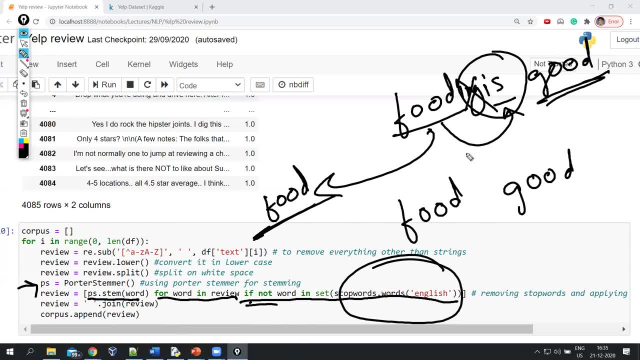 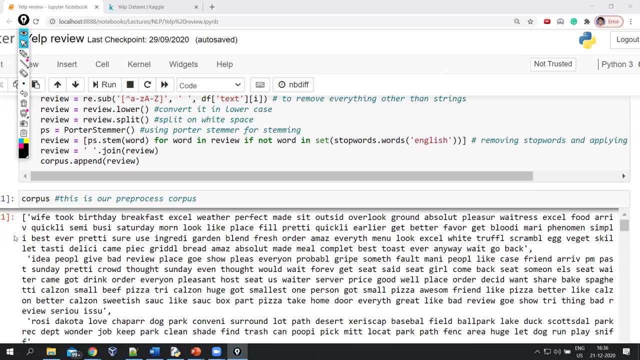 we will get a new sentence that is food good, which is in lowercase. punctuations are removed, stop words are removed and stigmatizing it is done. all happen due to this simple line of code. okay, this is the starter part of starter pack of nlp. okay, so you can see this. 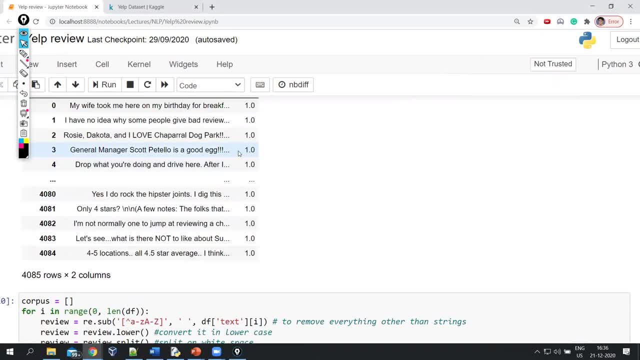 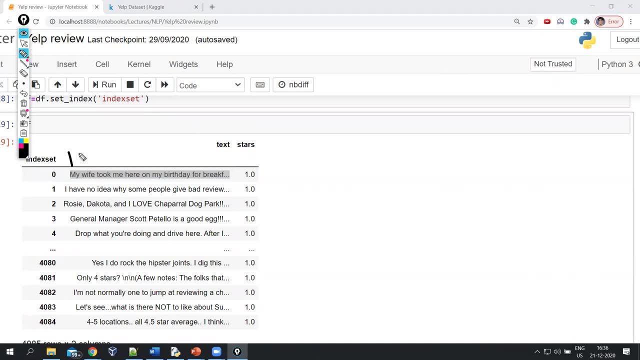 statement which is: wife took birthday breakfast. so my first statement was- i am explaining you in detail now- my, my wife took me here on birthday, so you can see my wife took me. so here, my is returned, my is removed. only what we have let his wife took me is me is removed. here is removed. 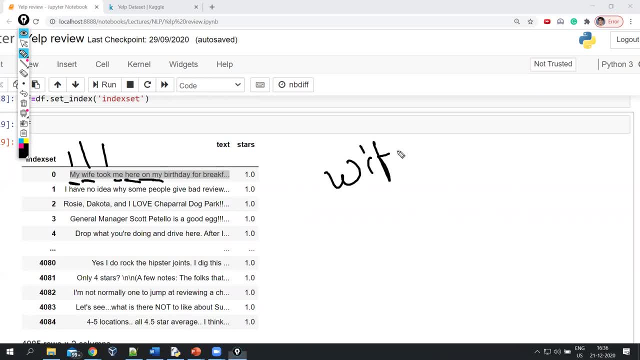 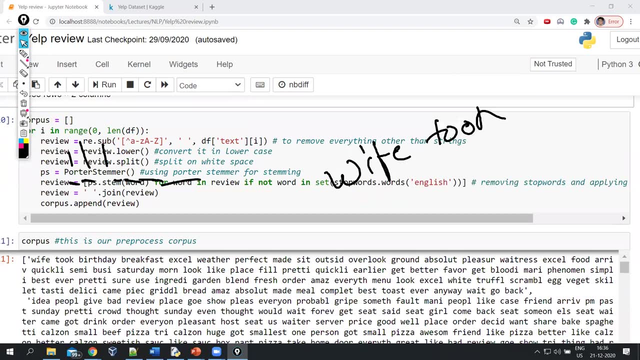 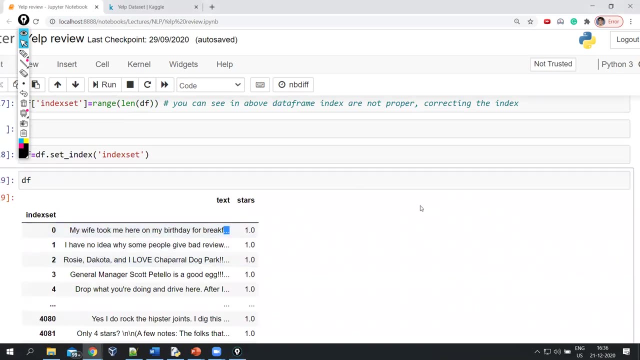 or is removed. my is removed, so you what you got. wife took breakfast, birthday or birthday breakfast, so the same thing you can here. wife took birthday breakfast, so it would be a complete sentence. only a small part is visible here because it is a long sentence. okay, and is it a positive or negative? remove. you can see that as. 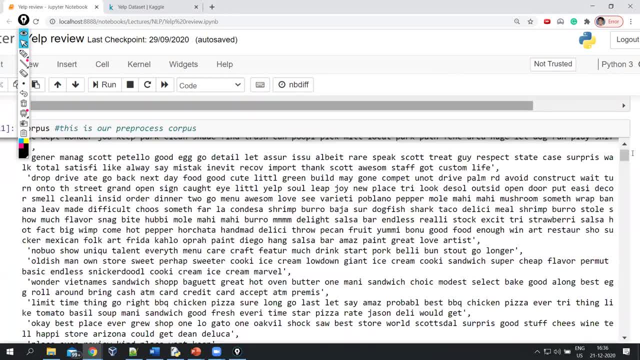 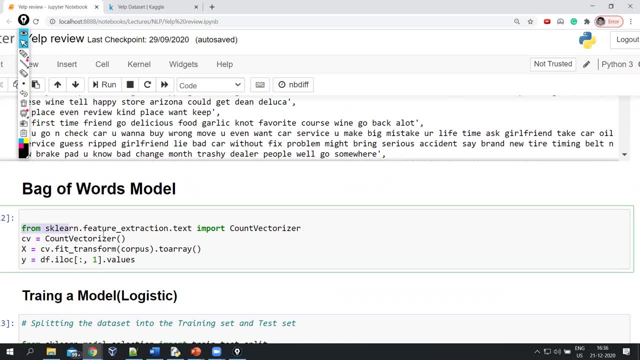 well. so in this way we have pre-processed our corpus. now it is ready to give to bag of words model. so it is very simple: in bag of word model you just pass. so this is your count vectorizer. you just use this cv count vectorizer function. you can export it from sklearn library feature. 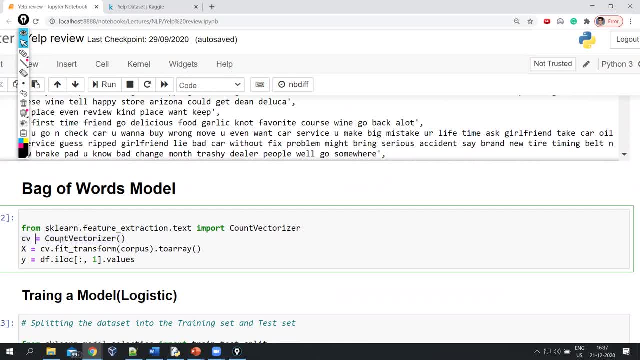 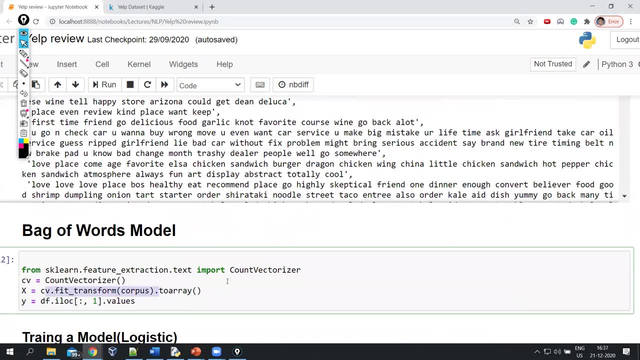 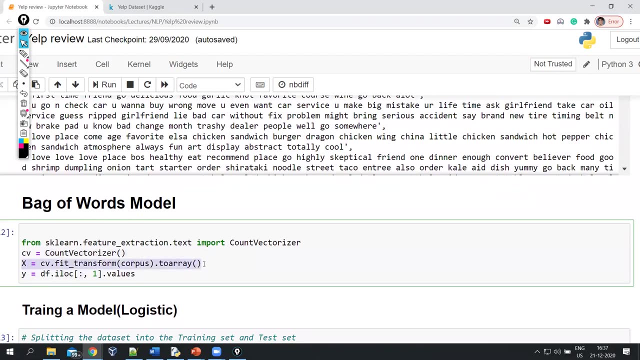 extractiontxt and count vectorizer. so on count vectorizer, i will fit. transport my corpus. so this is my newly generated corpus, which i have shown you. convert it, i will convert it into an array and then i will give this as a x. so these are my x features, this complete corpus, this bag of words. 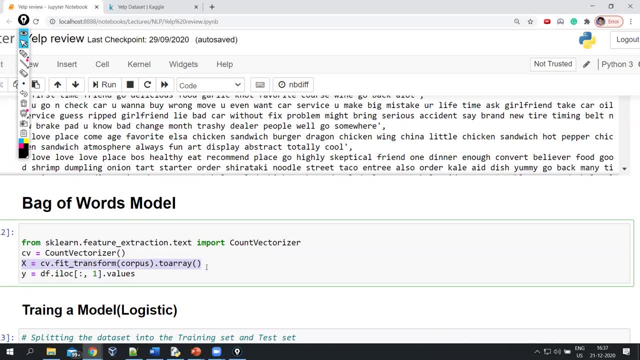 the same way, like i explained you, i will show you at the end how it looks like as well, how a bag of word, of models. you can visualize that as well. so it has created a bag of word models, and that is simply what it will have is first you have 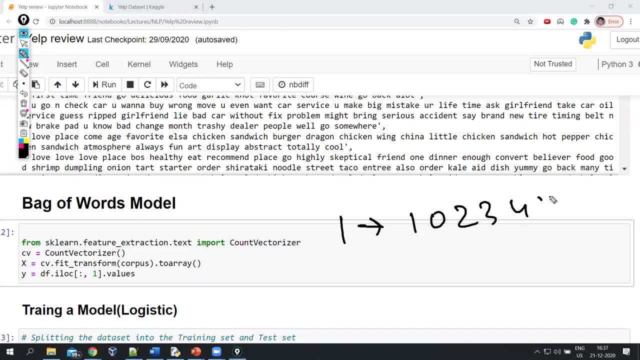 document one. so it would have some integers, some in this way, based on what are the unique words here. okay, so this is first document. second, in this way we have an array here, complete in the x and in y. we have whether it is a positive or it is a negative. in this way we have in x and y. so 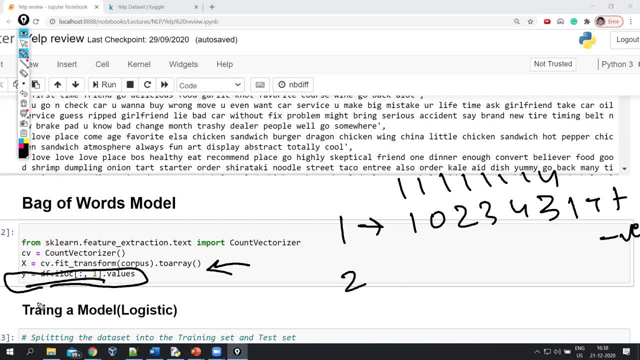 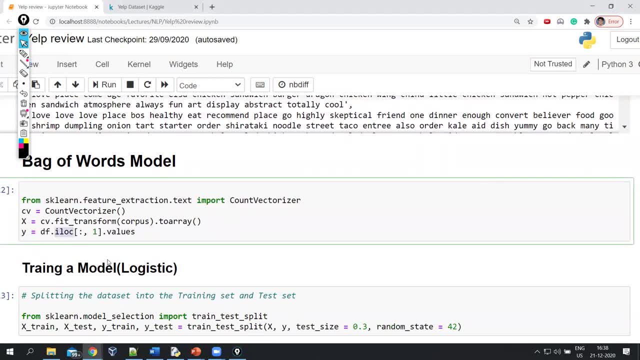 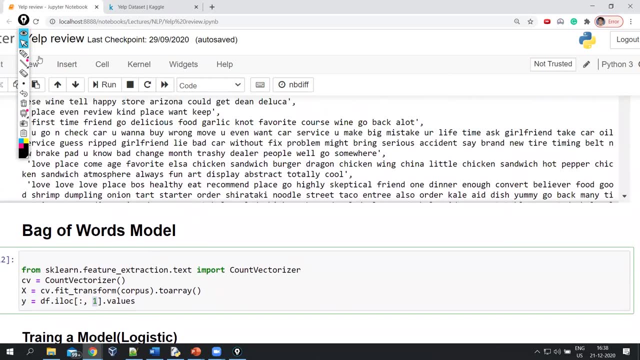 this is the code to extract the values for y. okay, so it will. i lock it for to get a particular indexed column. so i am taking the first column. okay, so naming starts in python convention starts from zero and one. so this is your data frame. for example, in zero i have here text and in one i have positive or negative values. so like you can see, 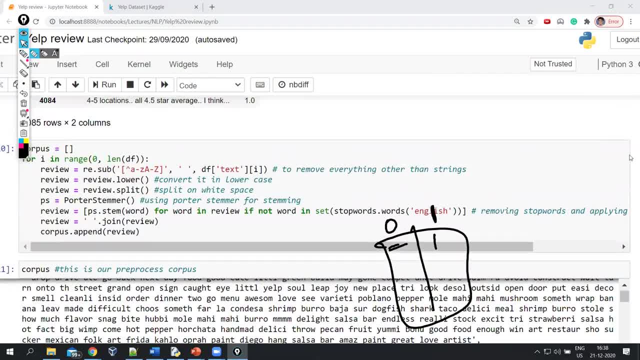 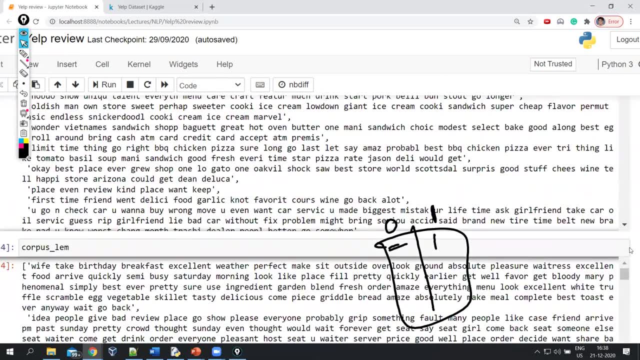 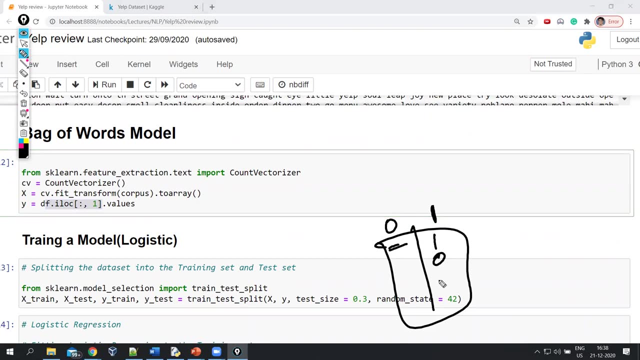 that as well, where i have lapped here, how much data i will take and start from my column. now let me let me see whether you have negative or positive, call it something like that. so what will i do here? so now let me introduce my code first. so the code that i will be using for my code is this: 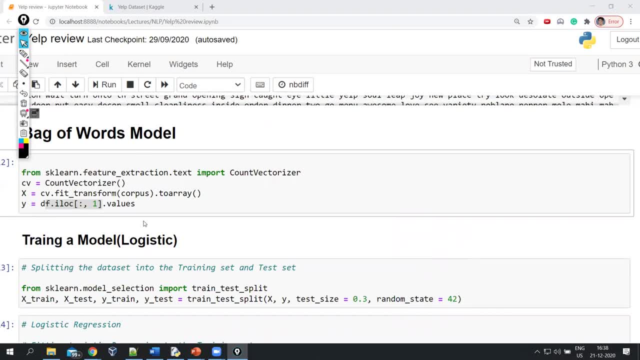 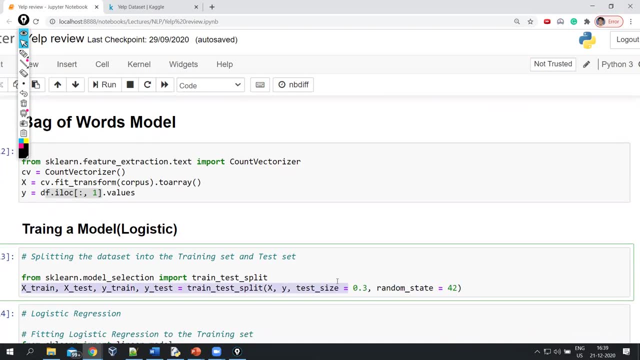 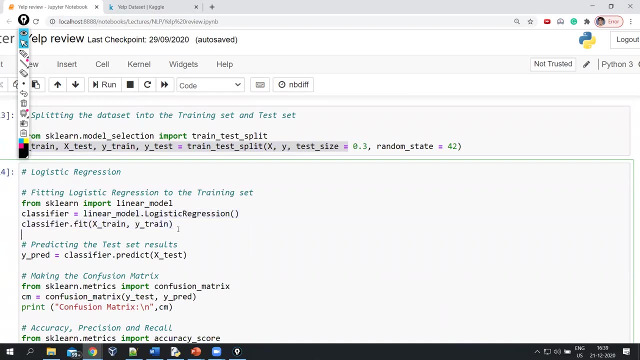 is my first, this is my text, this is my column zero and stars are my column one. so this piece of code which created a train test split which is 70, 30 of size, okay, and pass my training data set to my linear regression- sorry, logistic regression model, which will give zero or one prediction. 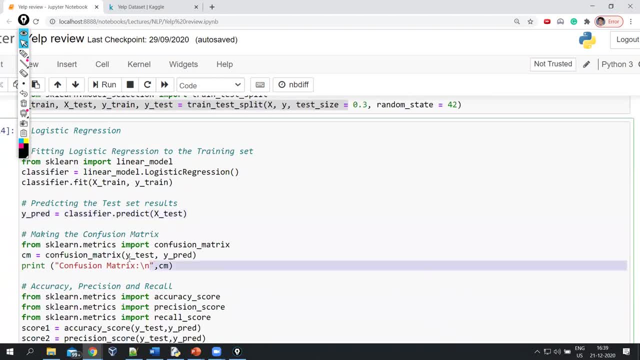 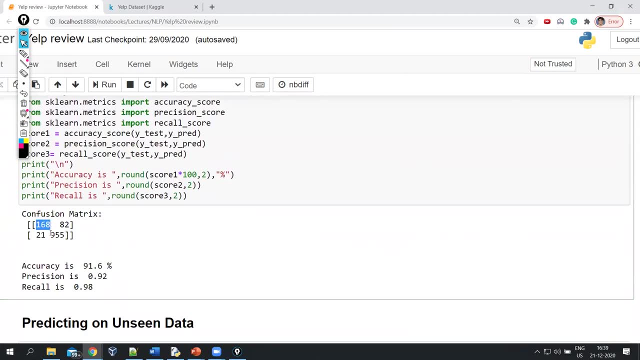 so after that i have predicted it and see i have seen the confusion matrix as well. so at the end you can see the confusion matrix. it has true positive for true negative. okay, false positive and false negative. so you can see my precision is 92, recall is 98 and accuracy is 91. 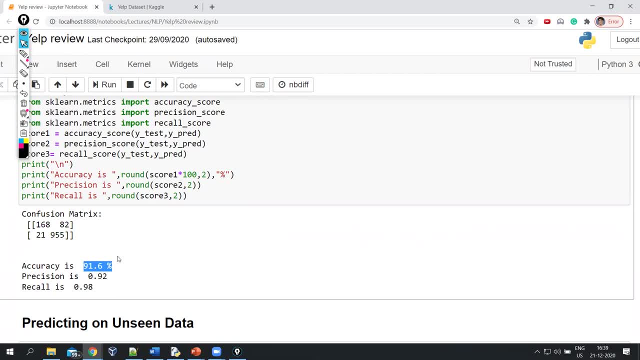 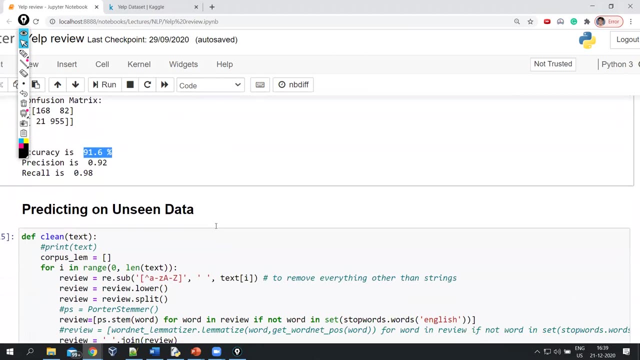 so if you want a video on this as well, you can comment it below. uh, if you want it for particular accuracy- what is accuracy, precision, recall or what is confusion matrix- i can prepare. just comment down what you want to learn. okay, if you want a video on logistic, i will create a video on logistic. 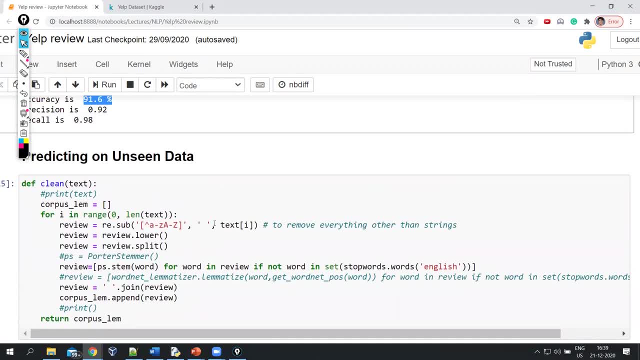 after that same thing. so understand this: we have created a data set and given it to model. now you can see that i have created a data set and given it to model. now i have created a data set in order to predict something from that model we need again to may give same type of data. 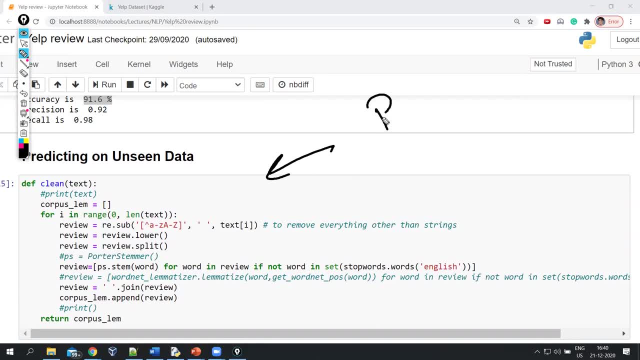 okay with same type of data means that we need to remove punctuations from it. remove punctuations then lowercase it, stigmatize it, after that convert. uh, yes, after that, uh, we can give that corpus to bag of words model. so, like, the bag of word models will create 1010 from it, like the integers. 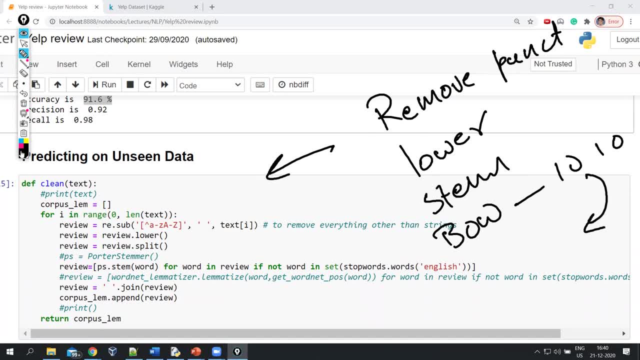 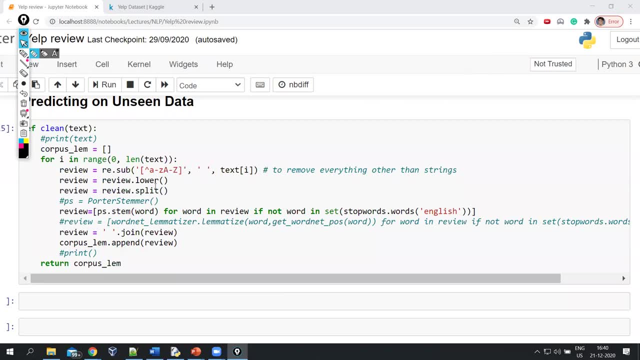 and then we can give it to our prediction model. so this, all things, are necessary to predict as well. on the unseen data: unseen is something: if a new customer comes and he gives the review, machine is able to predict it right or not, the same way i have done it here. so you can see i have used cv. 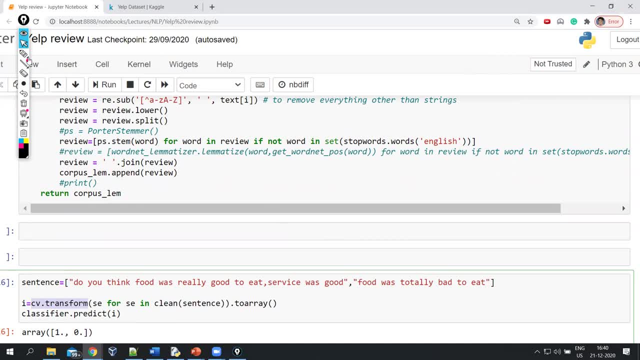 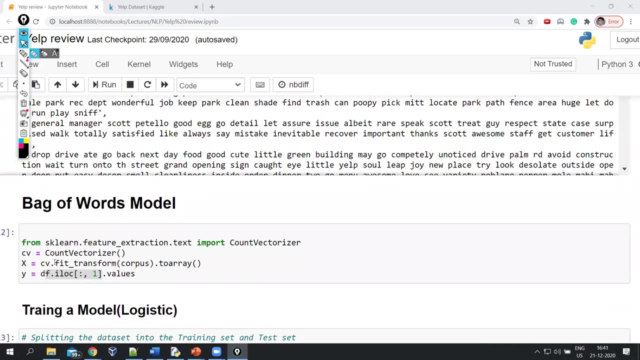 dot transform. so this transform what it will do. it has learned the features from using dot fit function. so, yes, so i have used here before this i have used dot fit transform. so if i show you bag of words model, i have used fit transform. so it will take our 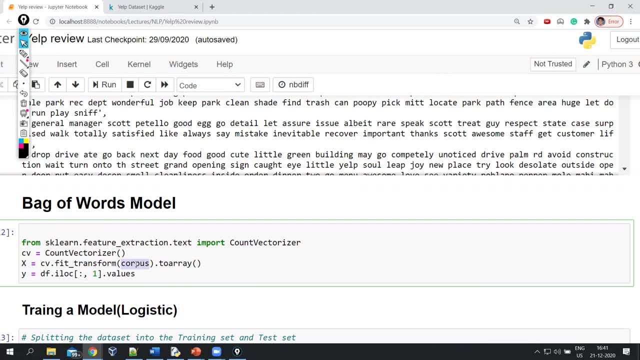 training corpus. this is called a straining corpus, so it will remember, or may it will remember, the unique words. like you food, so like i explained you, this words will be removed. remembered by the model using this fit transform. now, if you give a unique sentence to this, it will transform your. 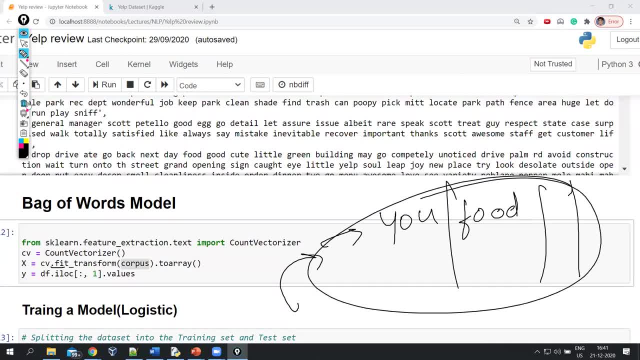 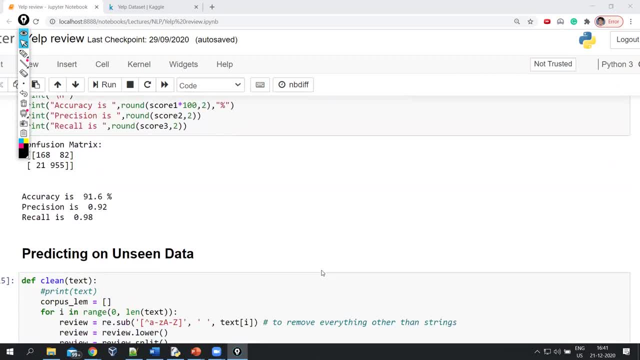 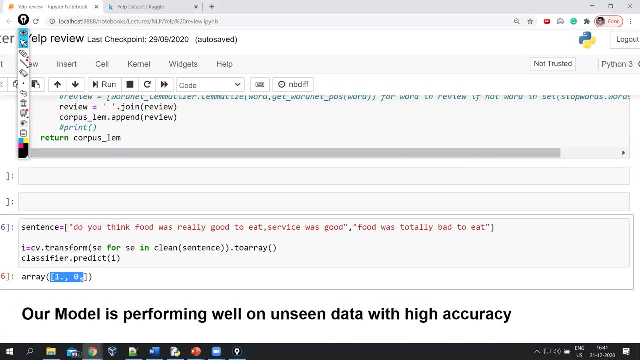 sentence based on this data. i hope this is clear. so, in short, you can understand that fit transform is used for training and transform is only used to predict the unseen data. so it will only transform the things, so it will transform and it will predict. okay, so, like my first sentence is: do you think the food was really? 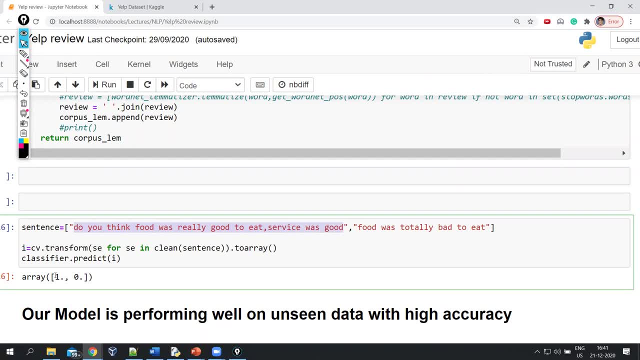 good service was good, so this is a positive sentence. i got one as a response. same way. second is food was totally bad to it. this is a negative review. so i got zero here, which is a negative statement. so starting from a simple downloading the data set to understanding. 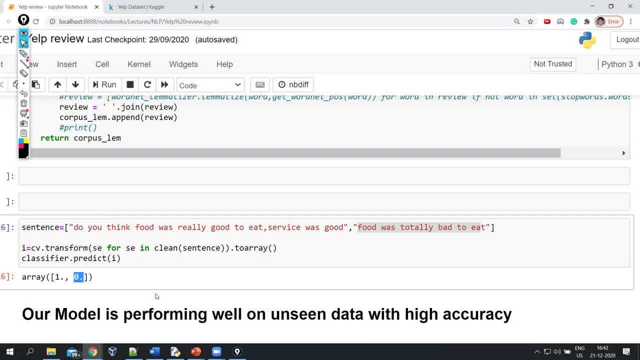 how to pre-process it and how to make a model learn on top of it, and then how to predict some something unknown to it. we have used a bag of words model. okay, so that is a complete case study on sentiment analysis. so you can give any sentence to it and it will predict for you. so i hope. 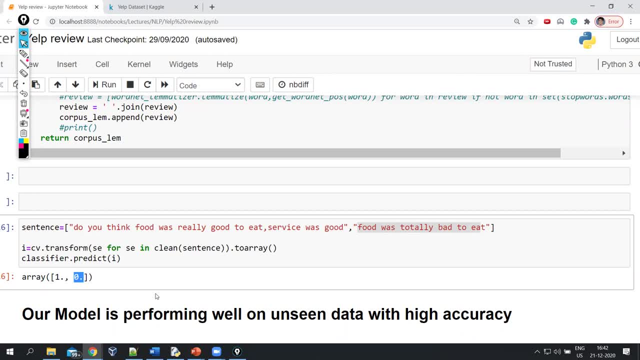 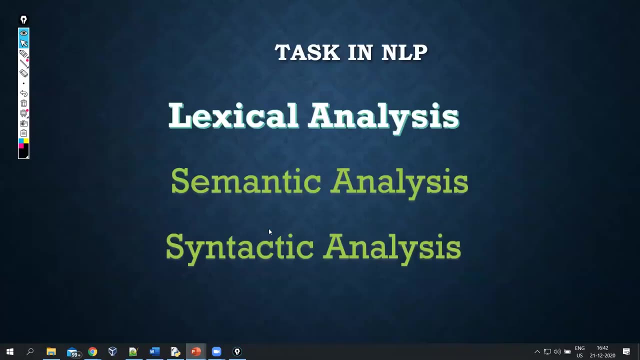 everything is clear to you if you want this notebook, so that is the only thing you need to do to get this notebook. jupiter notebook. okay, and yes, like i said you, i will show you the part that is bag of word model. okay, so how it look. 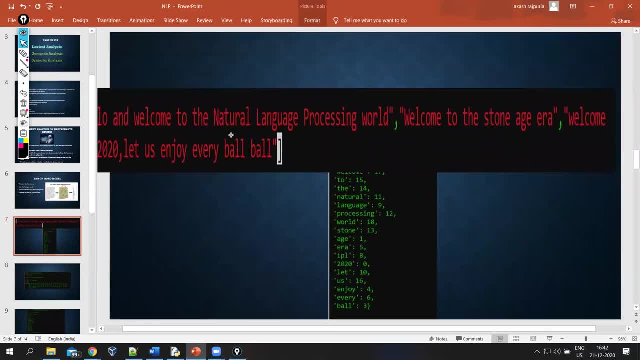 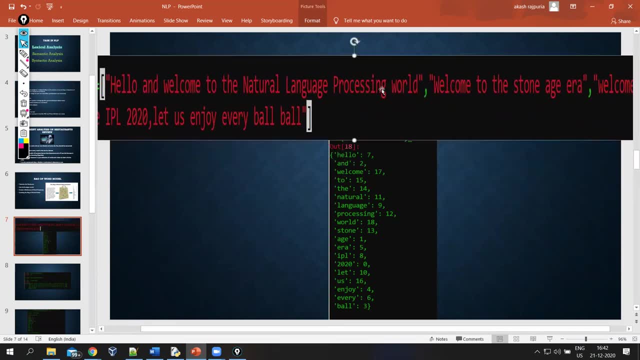 like. so, for example, i have this sentence. the sentence is hello and welcome. so everyone focus here. now i have the sentence hello and welcome to natural language processing world. so understand this now. i have been showing you just the last part of it: hello and welcome to natural language. 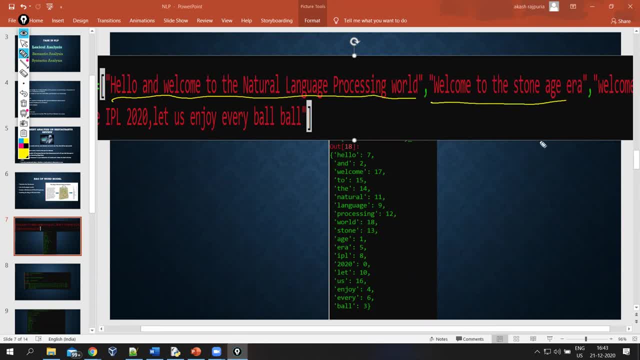 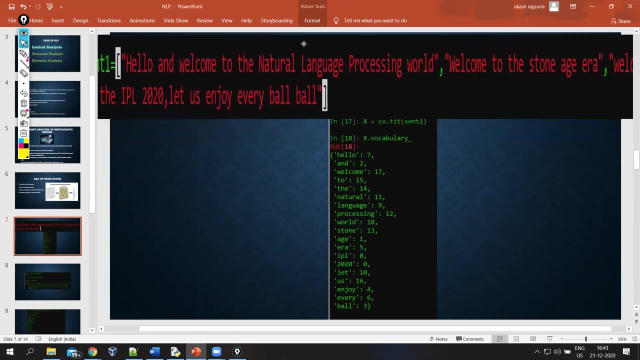 processing world. this is my first statement. second is welcome to stonejera and third is welcome to ipl 2020. let us enjoy every ball ball. so i have purposely taken this three sentence to explain you how bag of word models look like. so these are my three statements. 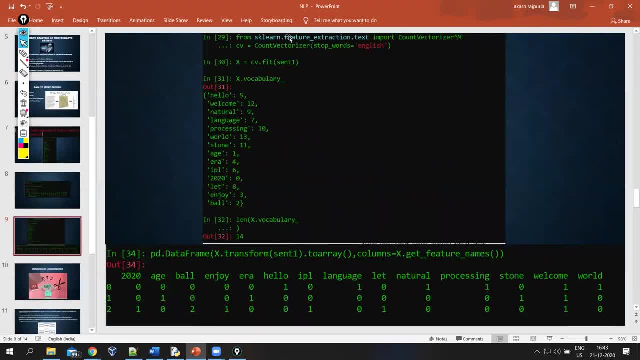 now same way, like i explained you, i will give this to my count vectorizer and fit it. i will remove the stop words from it and i will give this to my count vectorizer and fit it. i will remove the stop words from it and i will give this to my count vectorizer and fit it. i will. 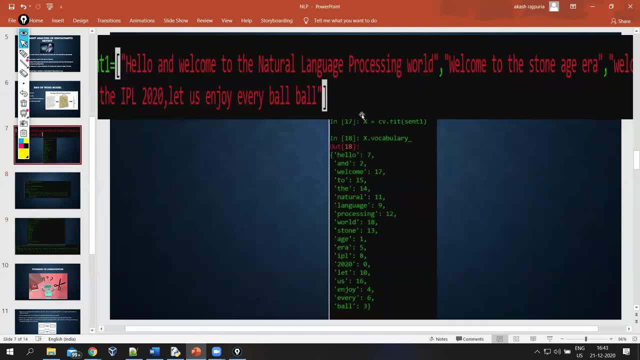 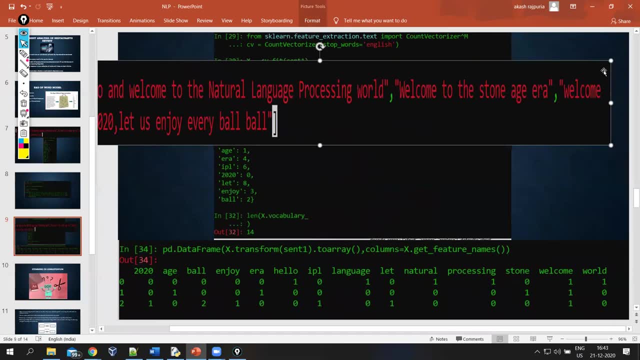 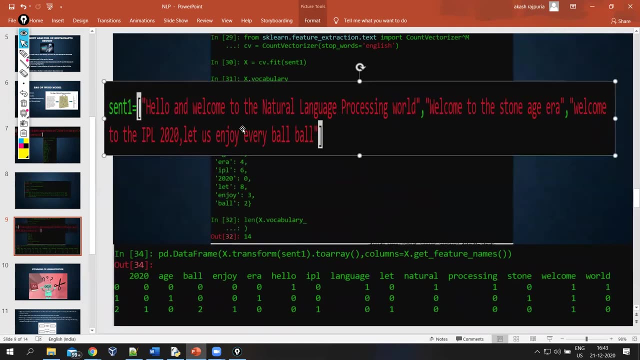 open this so you can see. so i would. i would do one thing for you. i will take this sentence from here and copy it here to explain, okay, so this are the same way. i have done all the things and you can see that now. hello, so each and every word from this. so, for example, 2020 age ball. this is after removing the stop. 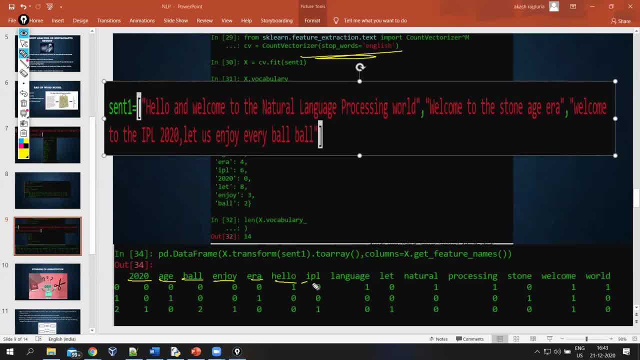 words. so enjoy era, so these are the unique words which are used in this scene item. you so enjoy era, so these are the unique words which i have created for you, that is, a bag of words model have created for you. these are the unique words all the so. this is my first document now. 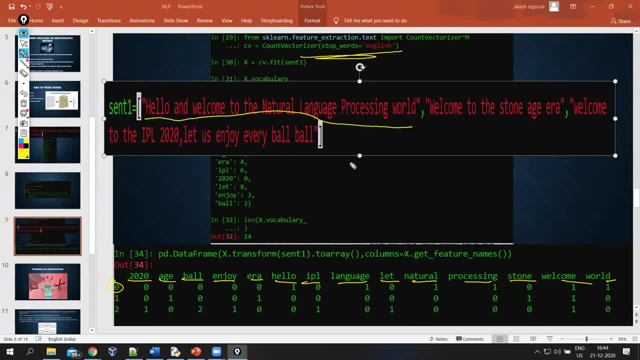 so, like the first document is hello and welcome to natural language processing world. so there is hello, there is no 2020, so i got zero here. then in the place of hello, i got one. okay, i will rub this and show you. in the place of hello, i got one. ipl is not there, therefore zero. then language is there. 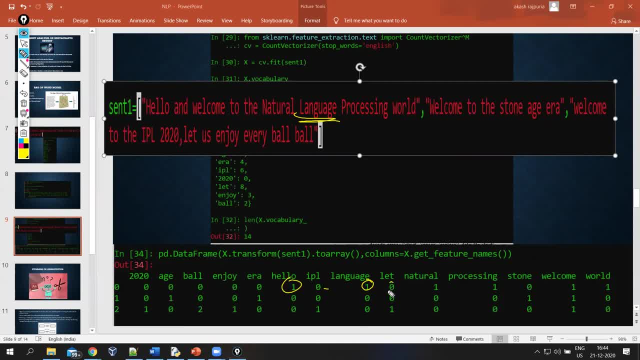 i got one here, same way. let is not there. zero natural is there? so one here? processing? is there one here? same way. world, is there one here? okay, so let's understand the third statement in that ipl is there, so i got for ipl. only ipl is present here, so ipl is only in the third statement, that is. 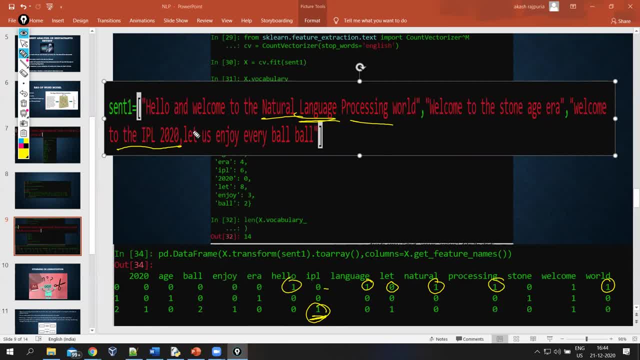 why i got one here. so same way now. so now you can see that in third sentence ball is repeated two times. so this is the first statement, first sentence. this is second sentence, the third sentence. so ball is repeated two times. so it will just count how many times it has returned. so now this is your complete bag of word model, and each 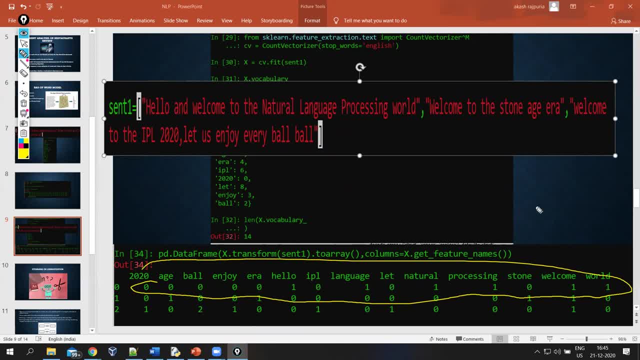 sentence is represent into the numbers. so you just give this number to the model. so, like i explained you before, so now you can see that in third sentence, ball is repeated two times. so this is your complete bag of word. ah, sorry, i forgot this one here. also in the third sentence, all the words. 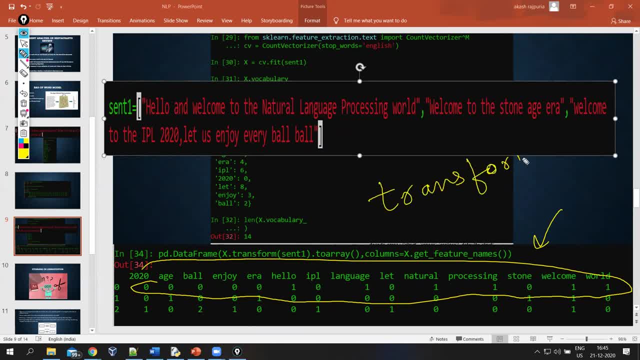 indicated in three words, that is, objects. that has in third sentence a value. if you use transform here, here now, if you give some unknown sentence to it and use transform on it, so it just transform it based on this vocabulary. it will not add some new word. if your sentence have a new word, it will not add it here and add the value. it will just try to. 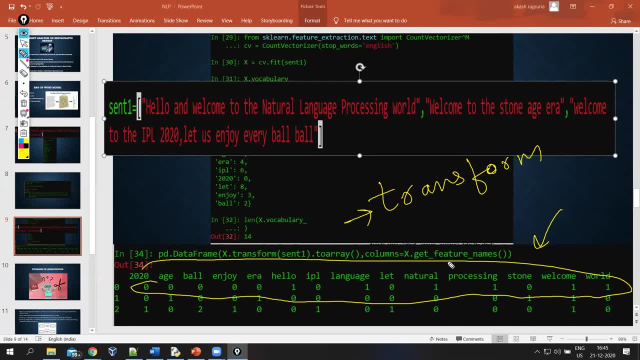 transform it between words. so if the word not present, it would be not there in this vocabulary. you will not get that word while predicting simple as ok. So this is about natural length, not language processing. i hope everything is clear to you. same way, like this is transformed, i have 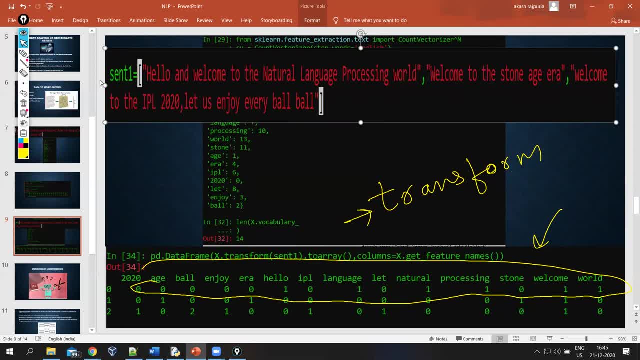 created a corpus in the same way with the pre-processing. so the sent one is our corpus. we have given to this bag of word model. so this bag of word models we have got for each sentence we have got some values and these values are sent to a model to predict okay. so that's all about. 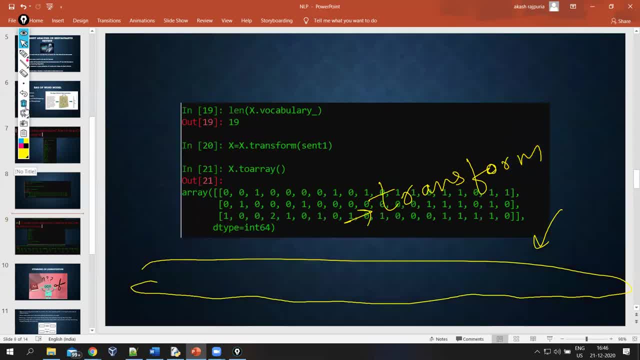 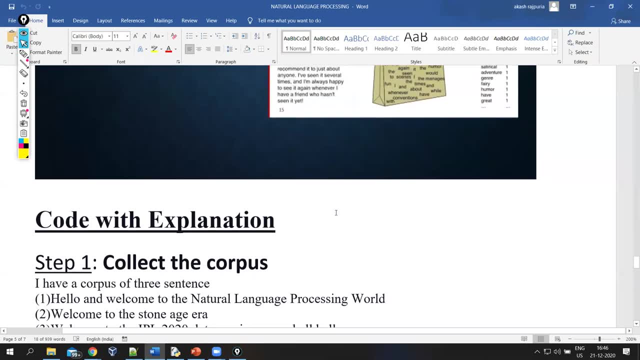 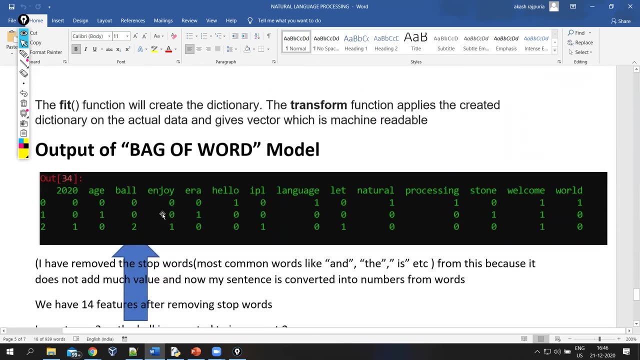 a complete natural language processing step starting. we have started it, so i will give you this document as well. if you want, just email me your id. okay, so this has a complete code explanation as well. this is the code which i have explained you using the fit transform. 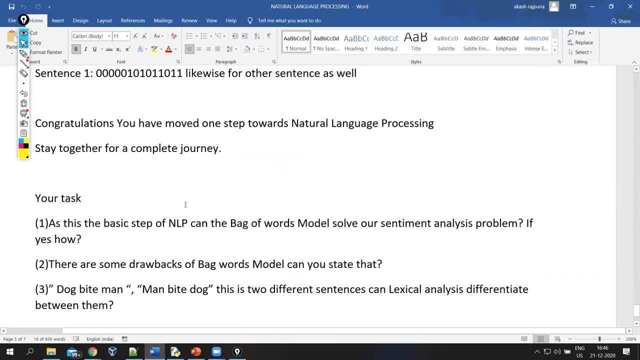 function. you can see the same code here. so bag of word model. okay, so that's all from my side. you have some tasks. if you want to understand that, just go into the deep or try to answer in the comment box. like there are some drawbacks in this model as well. so if you, 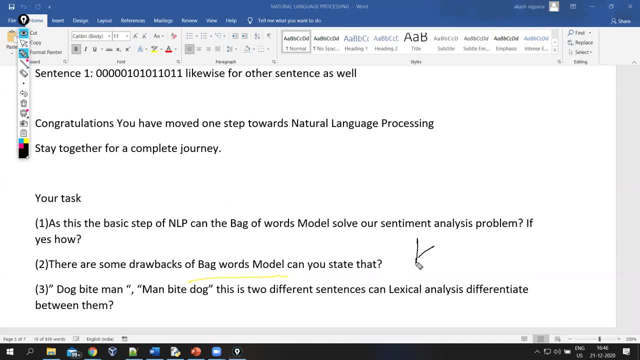 know that drawbacks. if you can identify that drawbacks, comment it below. i will reply you. okay, and one more thing. like you have a sentence: dog bite man and man bite dog. these are two different sentence, but can lexical analysis make that difference? you can understand that these are. 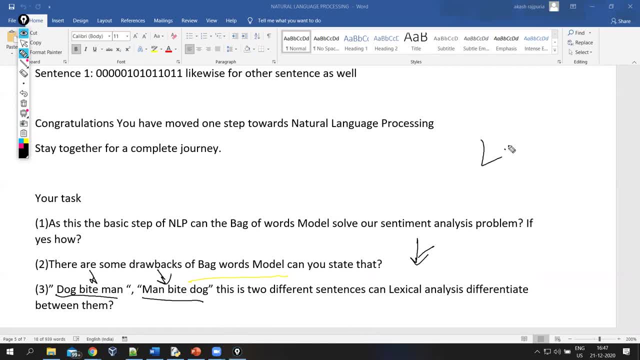 the two different sentence. but can lexical analysis? like i explained you, lexical analysis is tokenizing, so whether this can be differentiated using lexical analysis, comment your answer below. okay, so i hope everything is clear for you. uh, if not, just go to this video again. i hope everything. 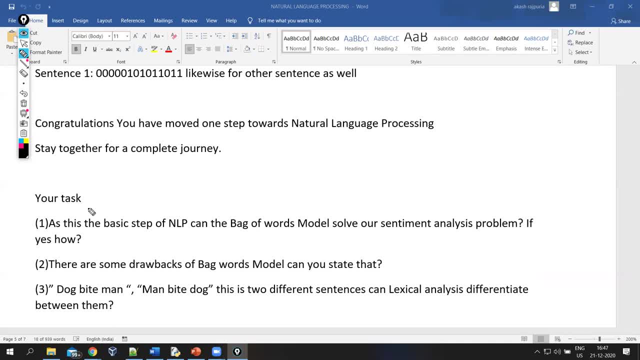 would be very clear. you can ask your questions in the doubt session in the in the comments below. i will be happy to reply you. okay, you. in short, this is the first step to nlp. now you have done first step. that is understanding, making a machine understand the norm, uh, natural language, that is text. we have seen the first step to it. 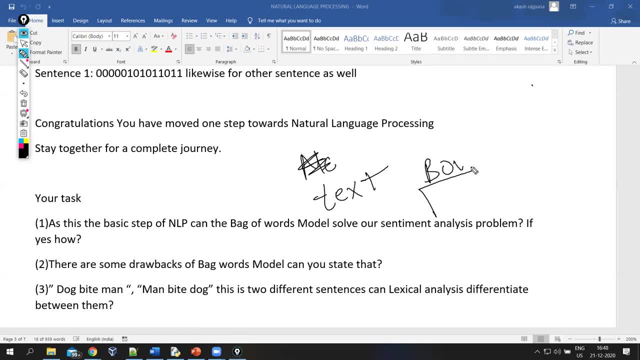 okay, first step. that is bag of words model. so if you like the video, spread it to your friends and comment what is your review on this. okay, if you want a particular video on some section, let me know and i will reply you. okay. so this is the first step to nlp. now you have done first step. 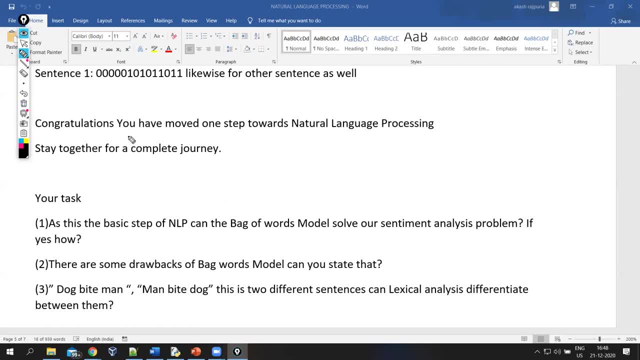 so i would be happy to share my knowledge. okay, so you can also share this knowledge by spreading this video, uh, to anyone who is helpful. okay, so till then, everyone, take care, we will meet soon. try to answer this question as your task. okay, this is very important to answer if you have. 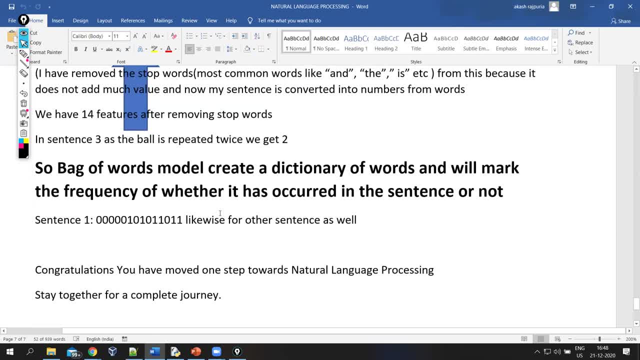 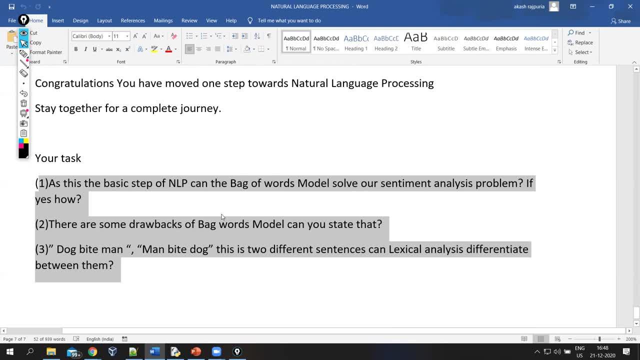 understood it. you can answer it simple as that, okay, so not. you can at least try it and i will give you whether the audio is good or not. i will give you the answer in the comment box. you are on a right track, or not? okay, so congratulations on completing first step. 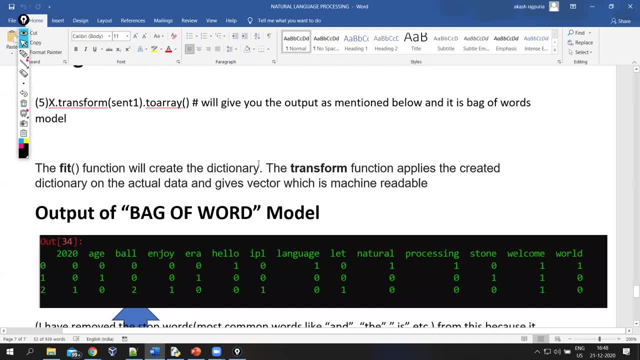 to natural language process. okay, if you want this notebook, comment your email. okay. thanks everyone. we will meet soon. till then, take care.